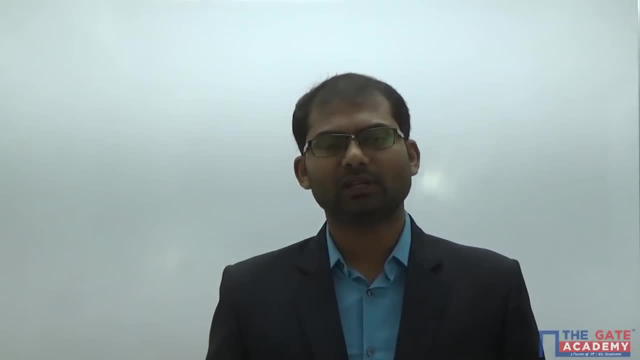 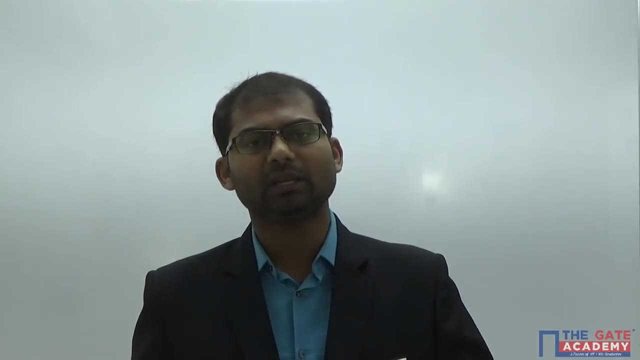 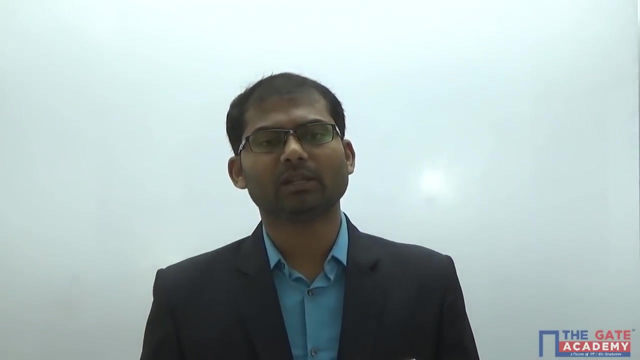 metal can take up to failure And this failure is actually defined as yielding in ductile materials and fracture in brittle materials. So because once yielding happens in ductile materials, we cannot use them. We stop using it Once the material which is a brittle material, 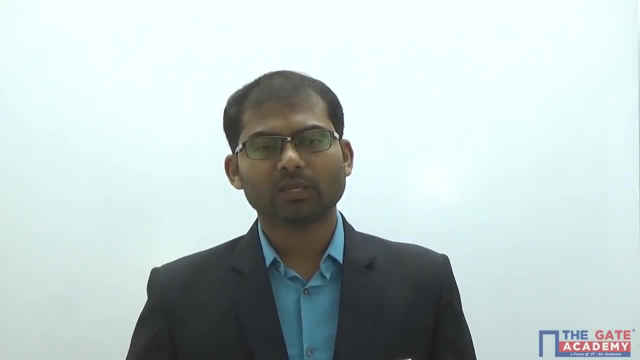 experiencing fracture, we will stop using it. So we cannot use a machine element once the material is going beyond yield point or ultimate point. So those two parameters or those two values are taken as strength of the material. Now, when you are going with 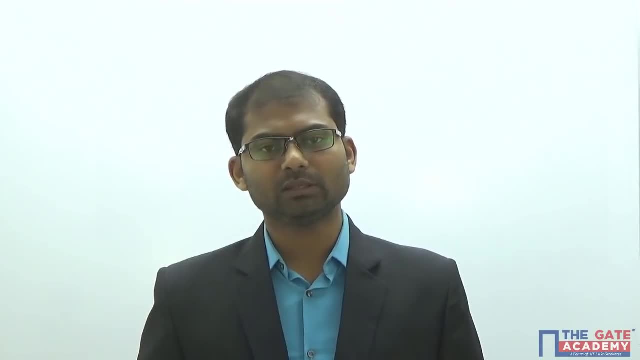 a particular strength. you can find out strength only in some loading cases. That means you take tensile loading or compression loading or shear loading. In those cases only you can find out the strength very easily, or you can decide very easily by doing experiment. 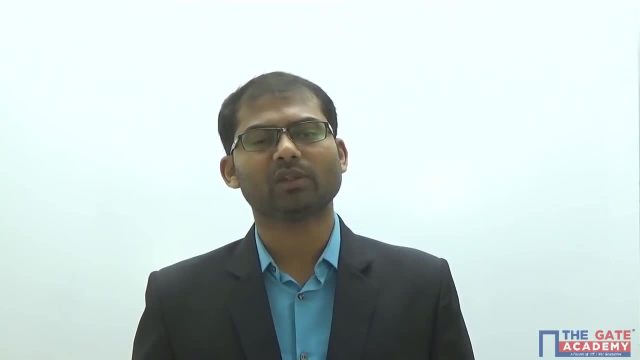 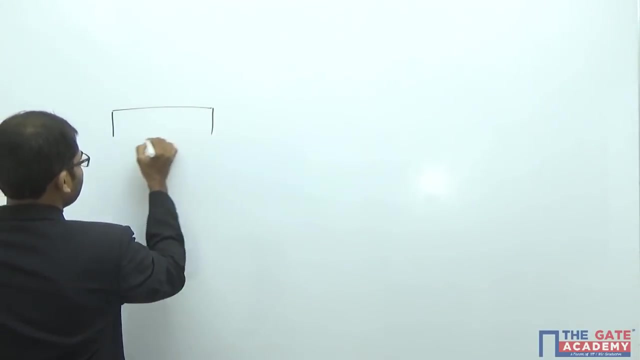 that, how much value of load will cause, or how much value of stress will cause, failure of the material. But if you are having a combination of loading cases, it is not actually possible. Let me explain you the earlier things. that is tensile loading. So if you are taking a tensile loading, 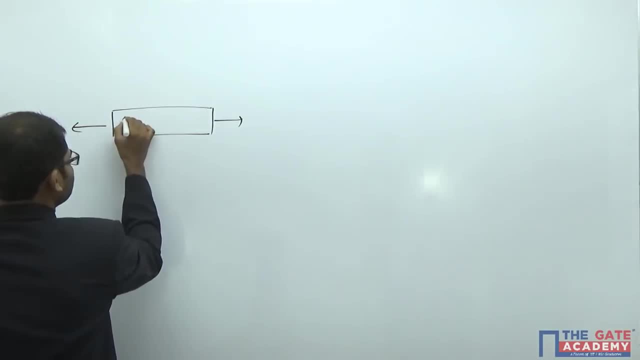 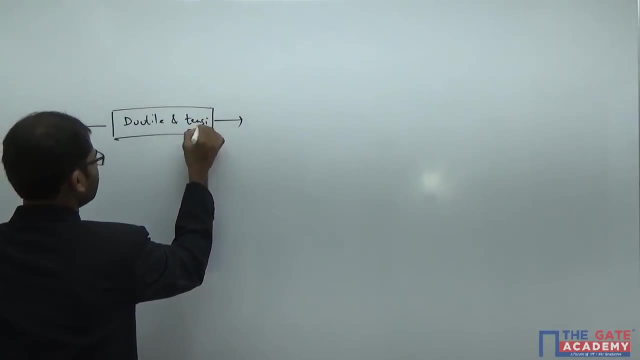 case, for example, it is a ductile material, So ductile and tension, or ductile material in tension. So here it will be corresponding to yielding, So yield point. I will denote it by S y t. Now, second one I can have. 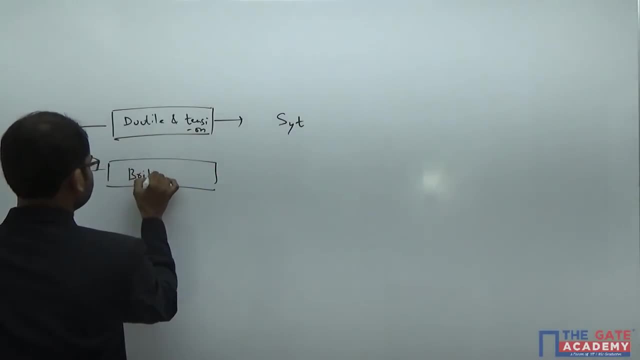 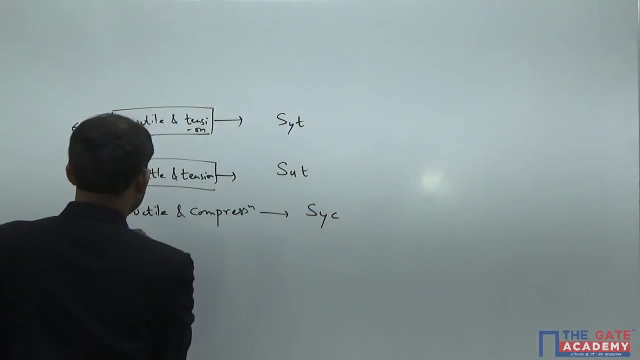 So a brittle material in tension. The dimension is S? u t because fracture happens in the ultimate point. So S? ut, I am denoting it here. In the same way, if you are having ductile under compression. So I denote it by S y c. Next one is brittle and compression. It will be. 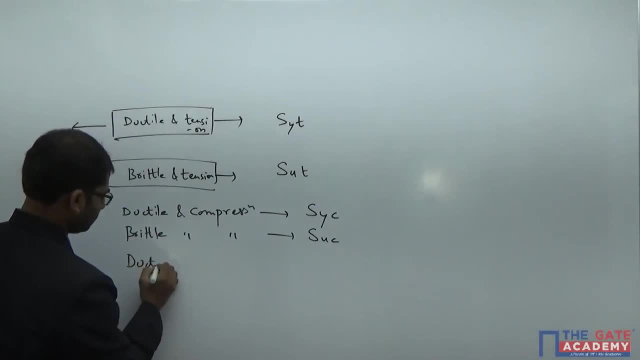 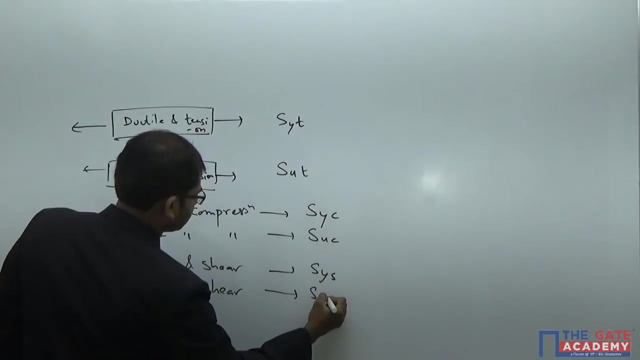 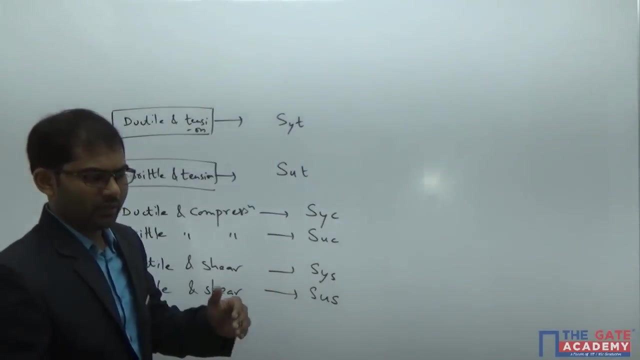 In the same way if there is ductile which is under shear loading Sys. so these values I can get by exponent. So once I get those values I can decide whether the upright load or induced stress will cause failure of the material or not. 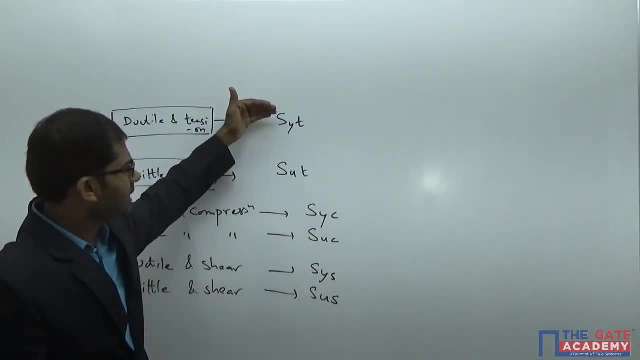 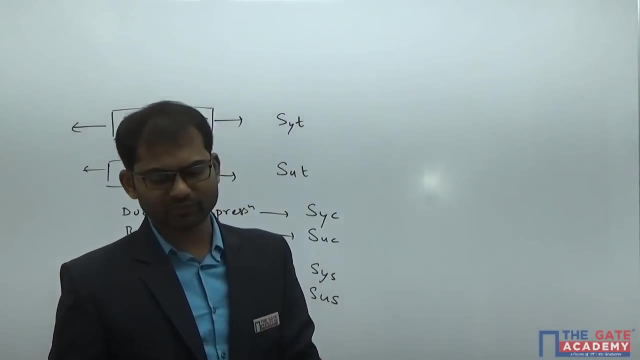 If it is more than this value, failure will definitely occur. If it is less than this value, failure will never occur. So in this case we can easily say so. in tensile loading I can say that if it is aluminum material, so for aluminum I will initially find out the value of strength in tension. 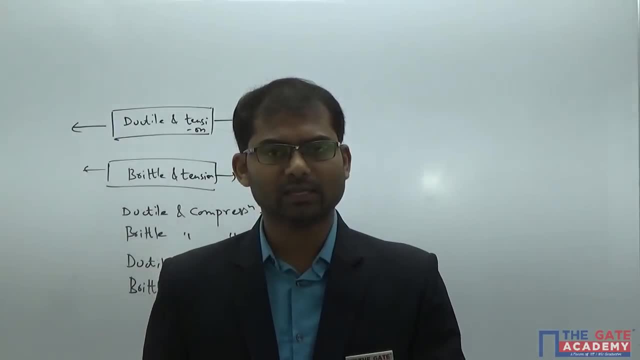 So if the load is creating a stress more than the value, I will definitely directly say that it is going to fail. If the load is giving a stress less than the value or the strength of the material, I will say that failure would never occur. 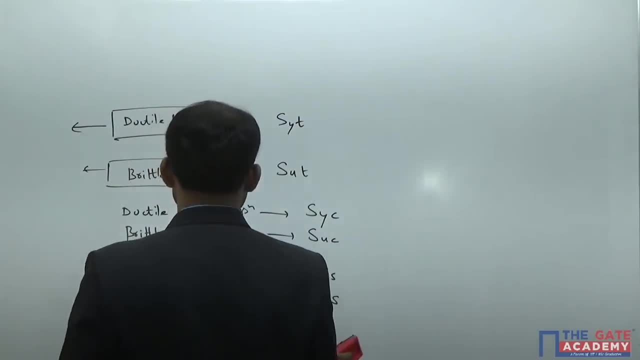 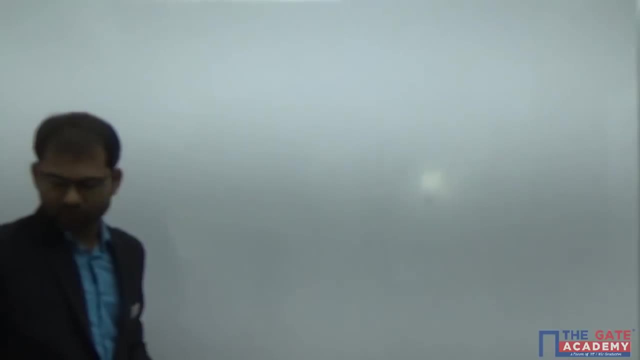 It is very easy to tell here. But when we are going with combination of loading cases, that means here every case we are having either tension, compression or shear, but not the combination of them. For example, we are having a combination of the cases. 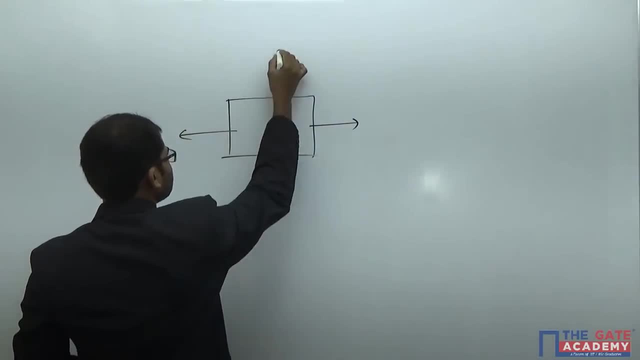 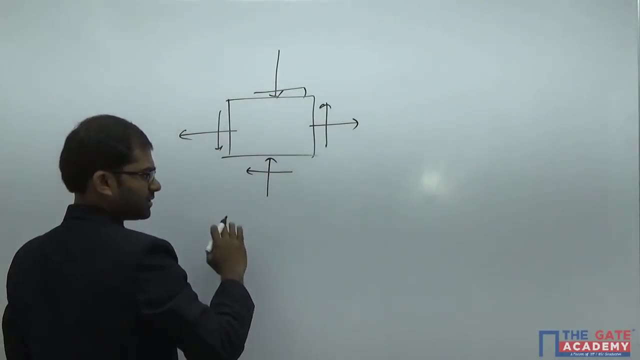 So we are having combinations here: the material experiencing tension, the material experiencing compression, also the material experiencing shear. So I took all the combinations here. You can go with tension plus compression, compression plus shear, so shear plus compression, like that. So you can take any combination. 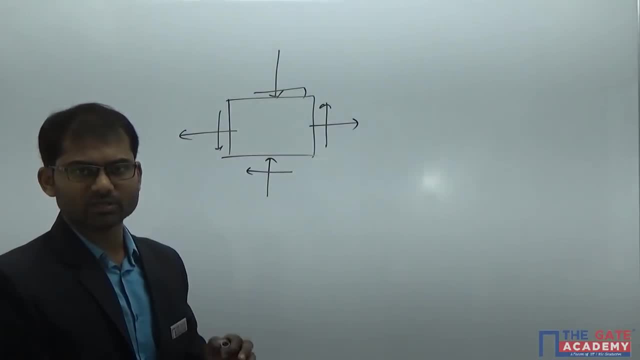 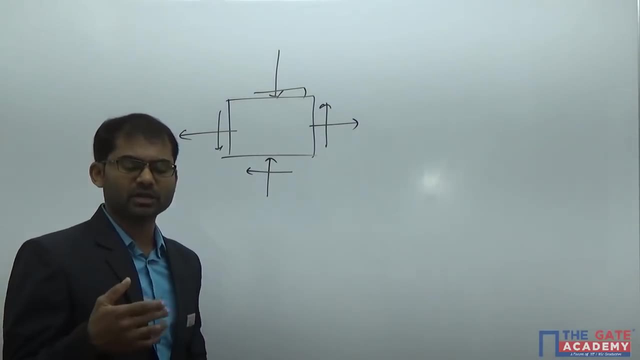 You can take a general combination of all these three loading cases: tension, compression, shear. So in this case you can't decide just by having those values. you can't decide that the strength, that means the material, will fail or not. 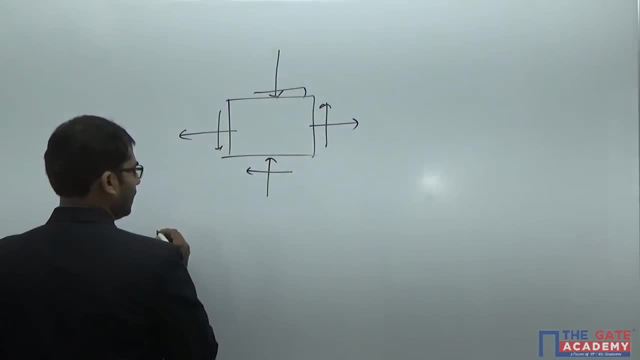 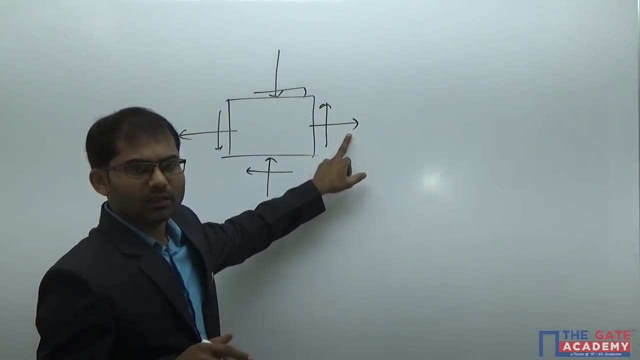 You generally think that if strength and tension is some value and this tensile loading is less than the value, failure would not actually occur by tension. If compression loading is more than the compression strength, it will fail by compression. We can't take individual values. 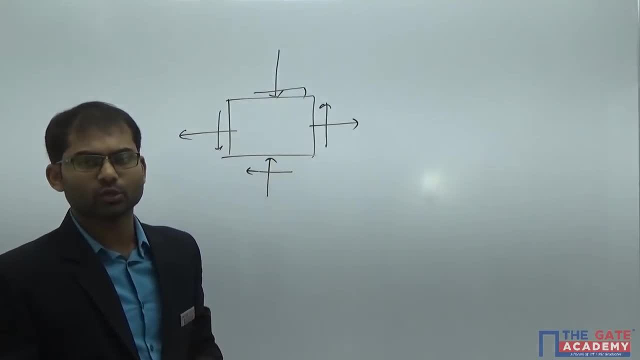 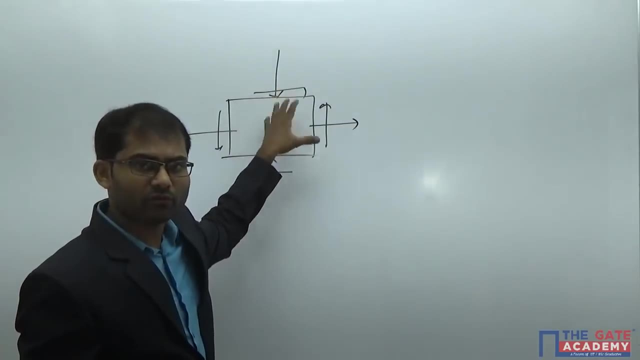 So generally our mind will tend to think in that way, but actually it's not true, Because when combination loading cases are there, the way the metal is going to fail is depending upon the effect of all these loads, So we can't decide simply by taking strength in only one type of loading case. 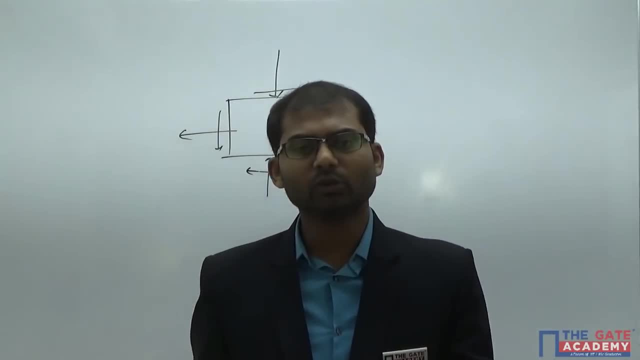 So to solve the problem or to decide whether the metal is going to be safe or not in these combination of loading cases. so we use theories of failure. So in general, everyday life, everywhere, in most of the cases we are having combination. 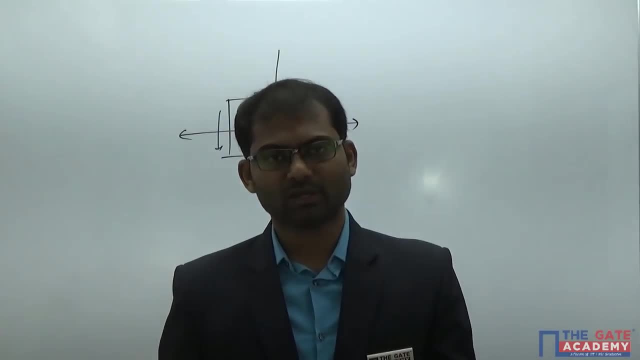 of loading cases only, either tension plus compression, compression plus shear, or tension plus compression, or tension plus compression plus shear. So everywhere we are having this combination of loading cases only. So we need theories of failure to decide whether the loads are going to cause or create or 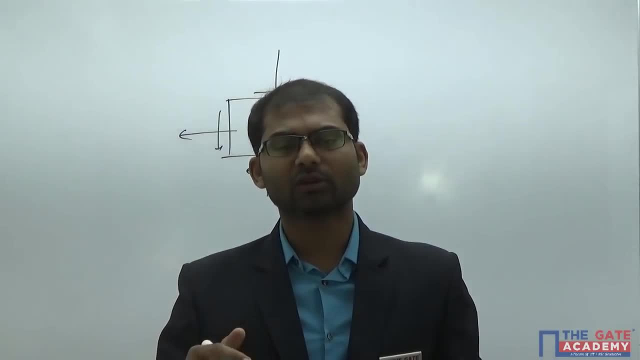 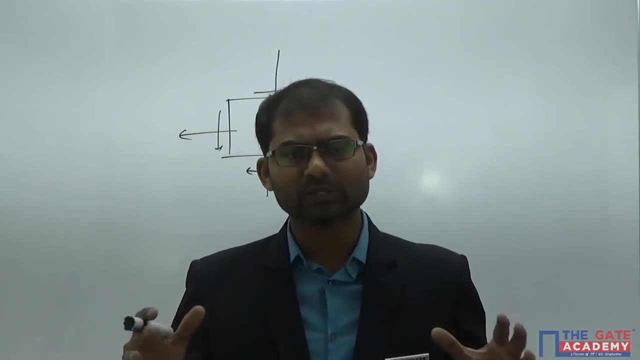 keep the material under safer conditions or not. So if the loads are going to create failure, so then we don't go with those loads. So we'll go with the decrease in the magnitude of load or removing some of the loads, or we'll do some sort of arrangement or some sort of modification. 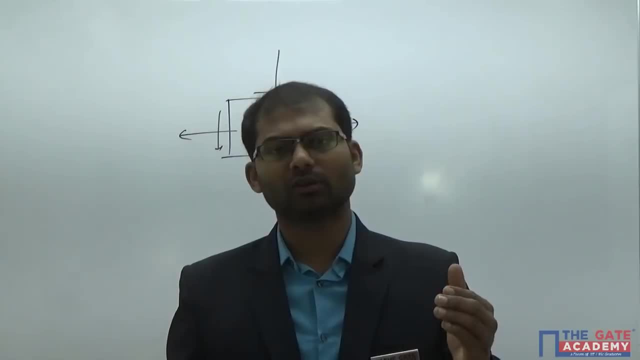 So that's the theory. So we're going to do some sort of adjustment such that the loads are not going to create failure in these conditions. So to decide whether the loads are going to create or the stresses induced are not going to keep the metal safe or not, we use, or we have to use, theories of failure. 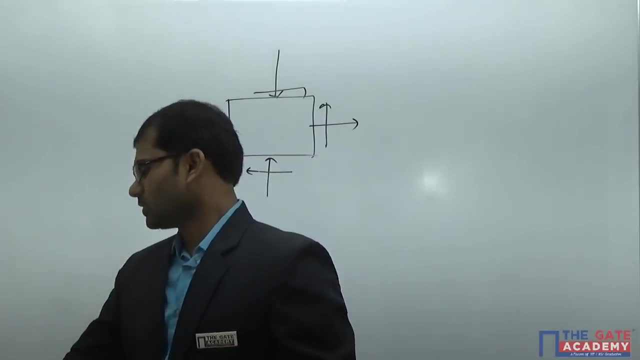 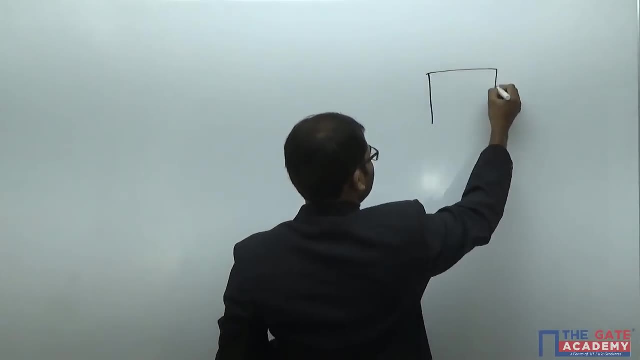 So I'll tell you the funda of the theories of failure here, or the basic principle by which we're going to decide. So we'll take the combination of loading case, whatever we're going to deal with that. For example, a general combination of loading case is like this: 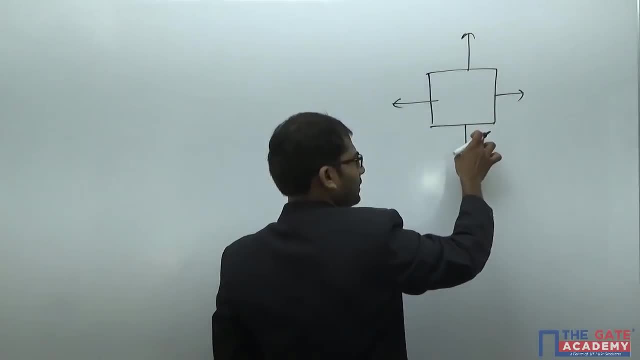 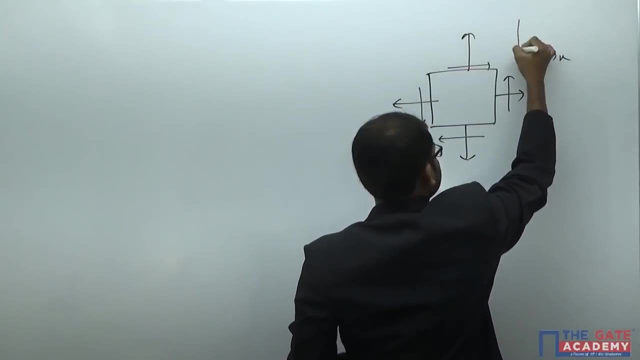 So tension in one direction, so I'm taking tension in another direction. here. this might become compression also, and shearing is there in the other directions. So if you take a particular quadrisystem, as this is x axis and this has y axis, so this 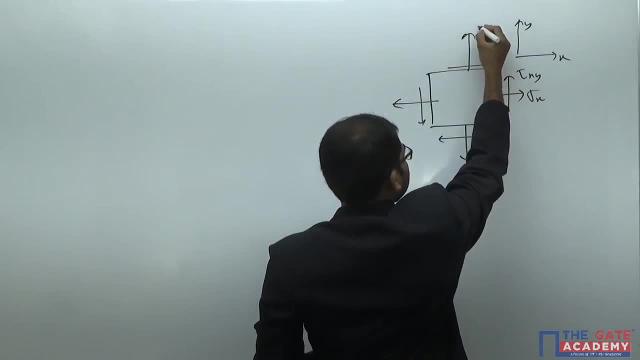 is nothing but sigma x, this is nothing but tau xy, this is nothing but sigma y, tau yx, sigma y, tau yx, tau xy and sigma x here. So we take the combination of loading case here Before going to the next part. we're going to take the combination of loading case here. 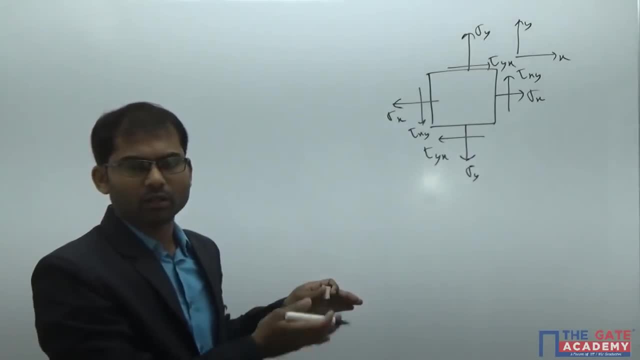 So we're going to take the combination of loading case here. Before going further, I should give you the list of all the theories of failure we're going to study, or basically, what are the theories of failure we should study for any complete examination? 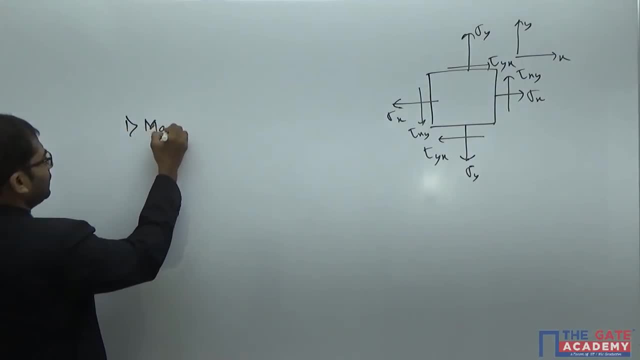 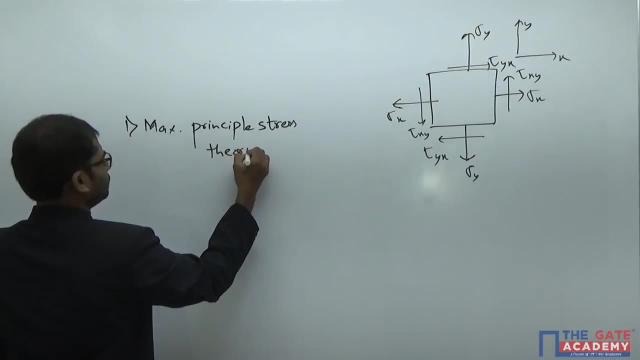 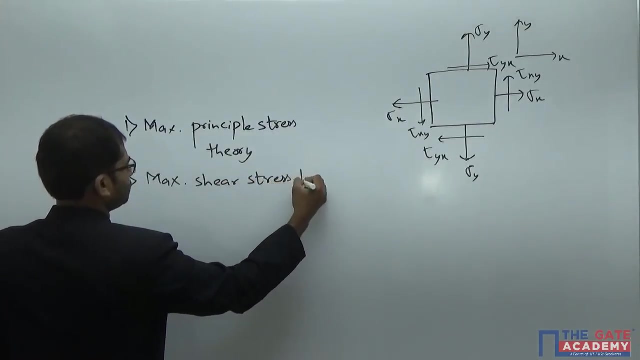 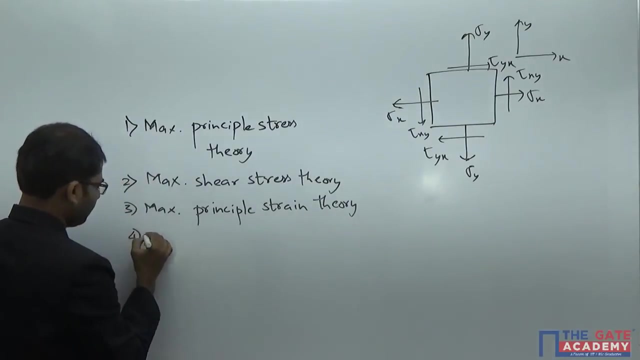 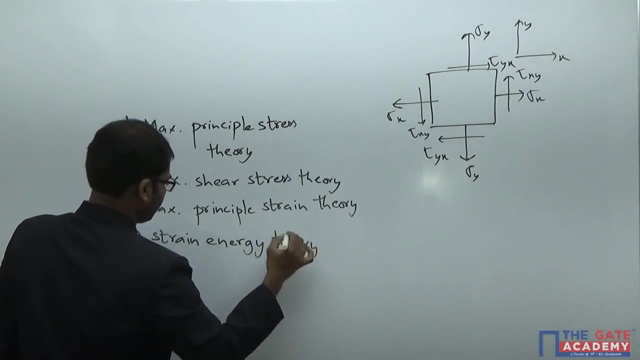 So basically there are five I've written down here. The first one is maximum maximum principle stress theory, Second one maximum shear stress theory And third one maximum principal strain theory And fourth one strain theory And fifth one is distortion energy theory. 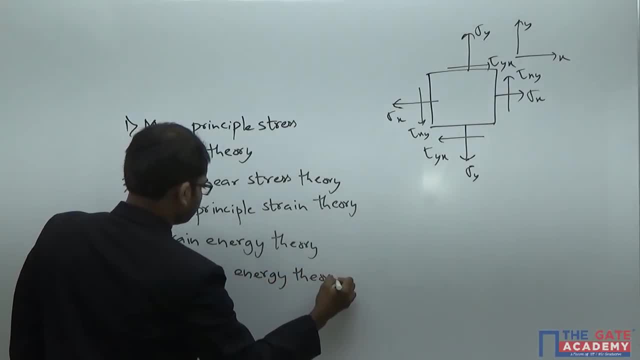 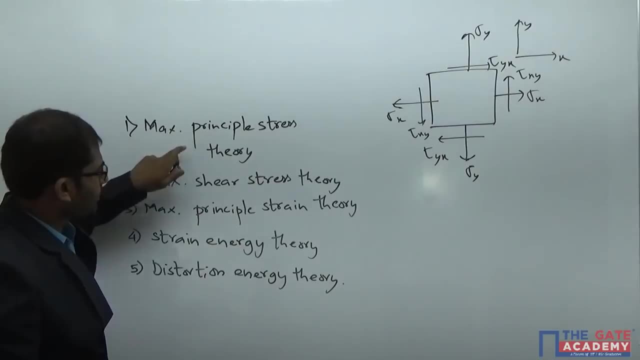 So these are all the theories, Okay, Okay, Okay. So these are the theories of failure here, and they're all given the names based upon a parameter: maximum principal stress, maximum shear stress, maximum principal strain strain energy or distortion energy. 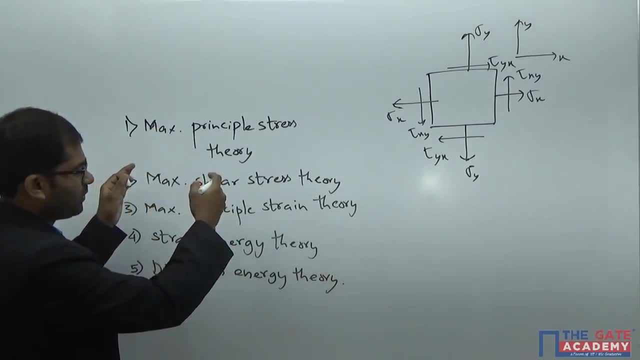 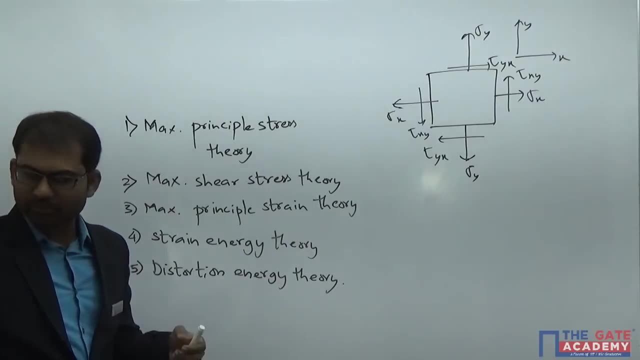 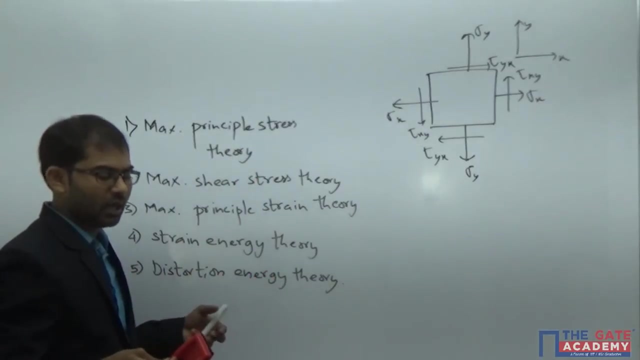 So the only calculations will be different because, based upon the parameter, the calculations will be done according to that, But moreover, the concept is the same as well. So we'll take this explanation part with respect to this maximum principal stress theory, and then I will explain you these two theories of failure so that you can understand how. 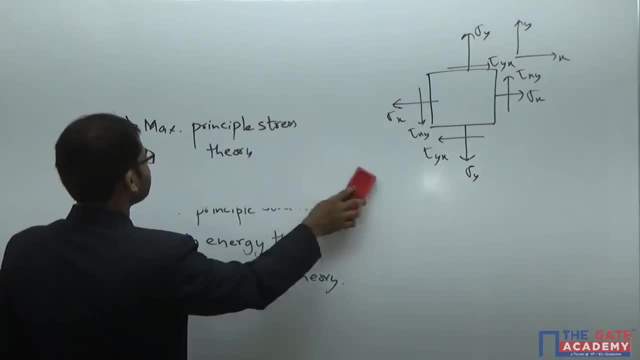 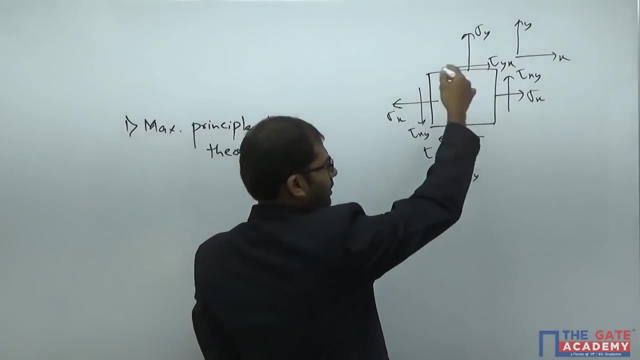 we had to apply the concept and solve the numerical. So first of all I'm going to maximum principal stress theory here. In this one the parameter is maximum principal stress. So for this loading case, based upon my strength of material concepts, I will find out the 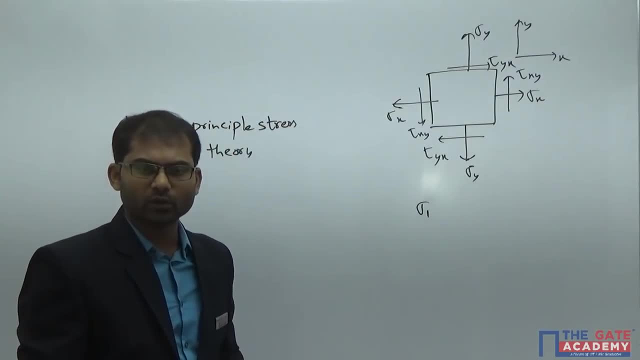 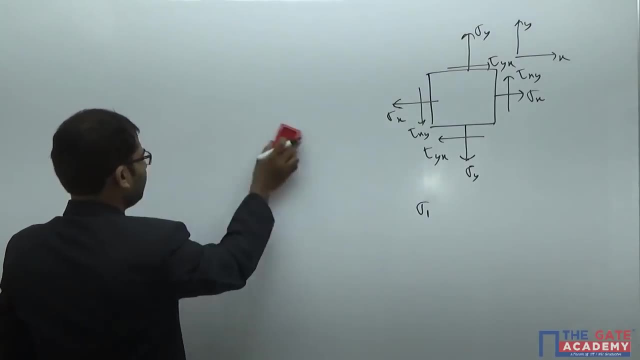 principal stress for this loading case here. So whatever will be our loading case, we can easily evaluate the value of sigma 1.. So once you get sigma 1 here, so we have to compare the sigma 1 with the sigma 1 in uniaxial. 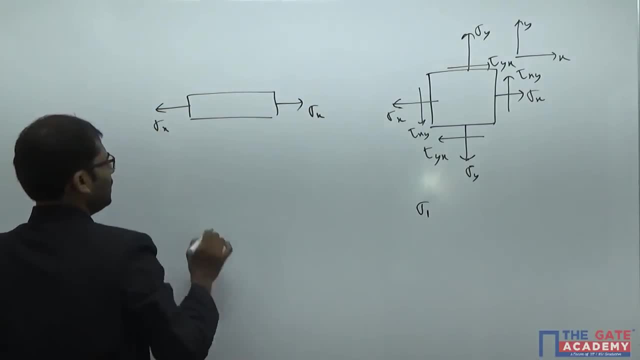 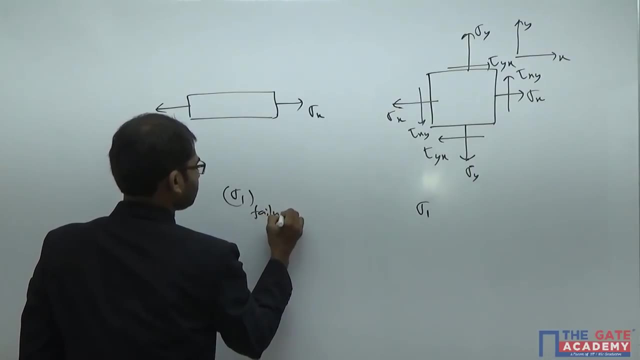 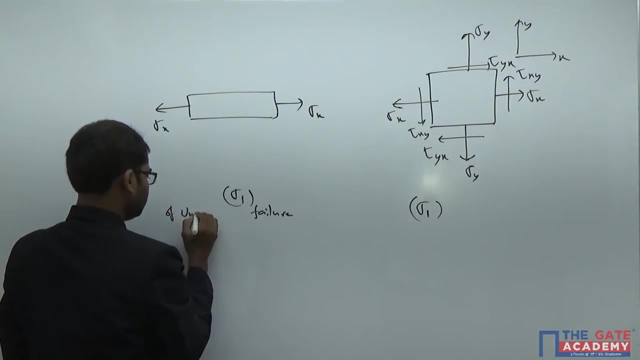 loading case. If there is sigma x in this acceleration here, So sigma 1 of this case at the time of failure. this combination loading case here and sigma 1 of uniaxial loading case, sigma 1 of uniaxial case. it is sigma 1 of uniaxial case at failure. 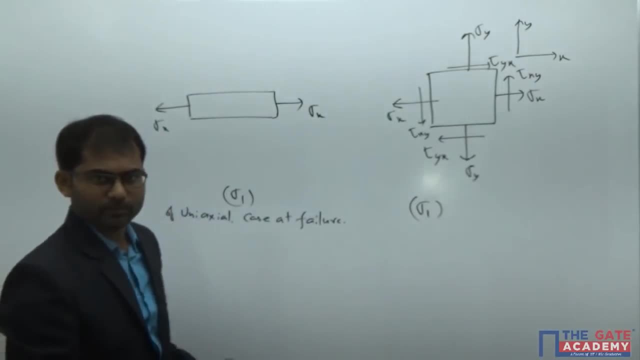 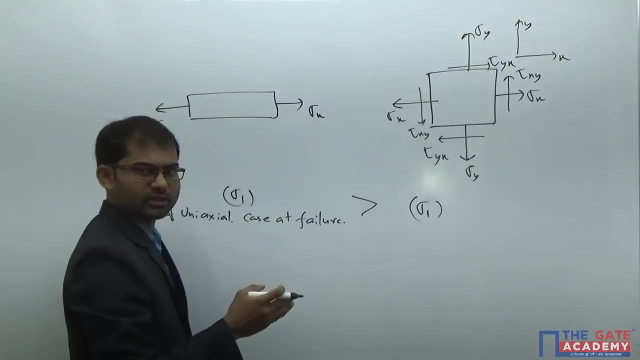 So the sigma 1 of our combination loading case here. So the basic principle here is: if our sigma 1 is less than this value, then it will be going to be the same. Every theory of failure is the same in its way itself. 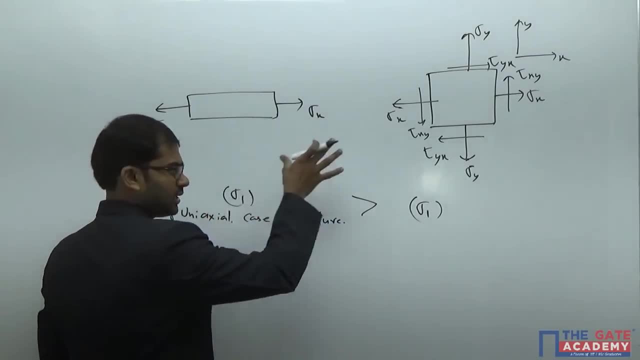 For example, if it is maximum shear stress theory, so here we will be taking maximum shear stress and here also we will be taking maximum shear stress of this case here and we compare. So our parameters should always come less than this value here. 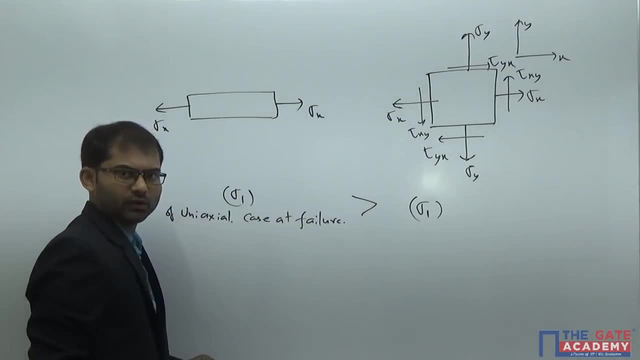 Otherwise you will be experiencing failure. Later we can check how authentic it is and it is valid. our particular theory of failure is valid. for how many times it takes? Ok, of materials, nothing we can decide, but basically principle of the each and every theory is: we have 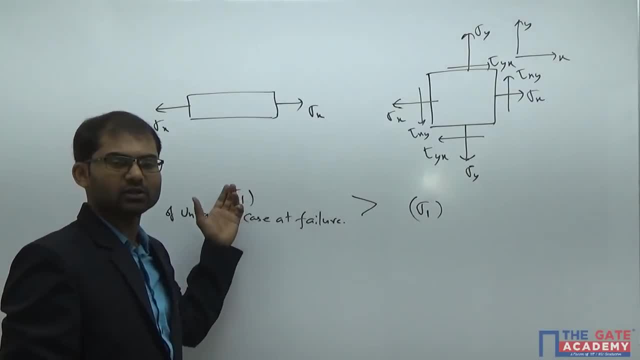 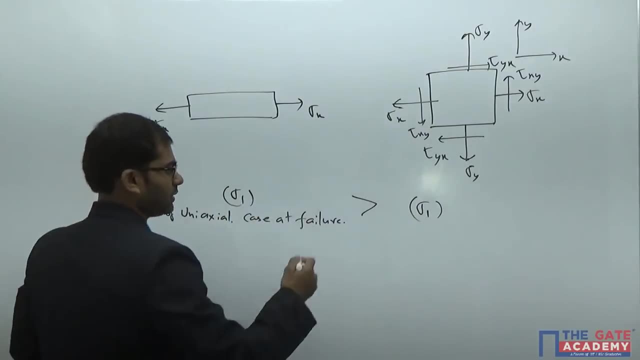 to find the parameter for our combination loading case and compare with uniaxial loading case. at failure, if it is coming lesser than this value, the metal going to be safe. if it is not coming lesser, it's not going to save. so this is this inequality: satisfied it's going to be. 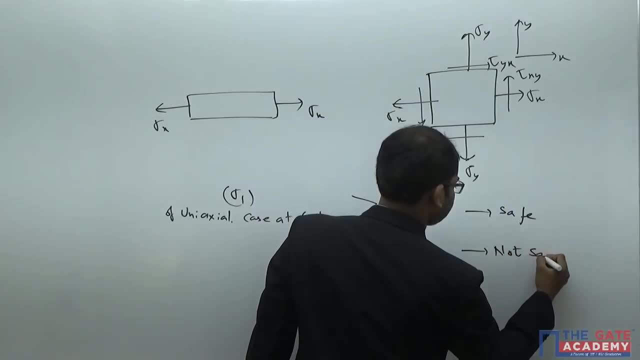 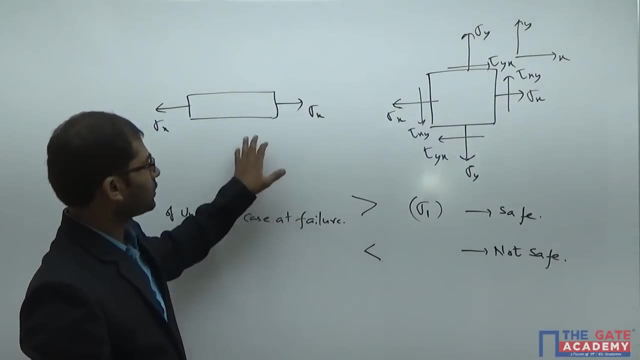 safe. if it is lesser, it's not going to be safe. it's not going to be safe at all. it's like this one here. so now, when, as we are comparing with the uniaxial loading case, first of all we should know, or we should analyze this uniaxial loading. 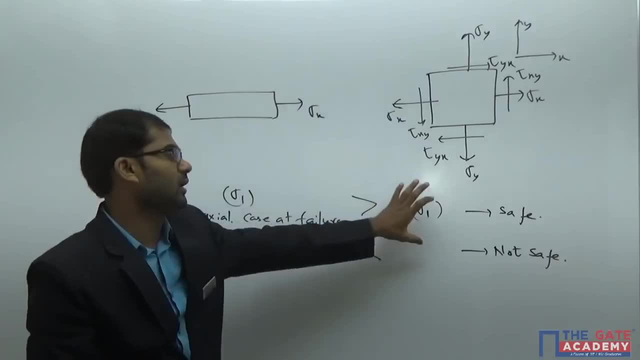 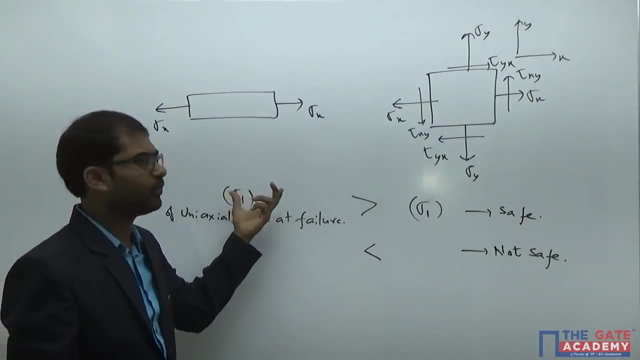 case clearly. then only we will be able to understand how to relate with this value, with this value here. so first we should know these values: sigma 1 or tom x value, or a principal stress value or strategy or anything corresponding to uniaxial loading case here. so first of all, 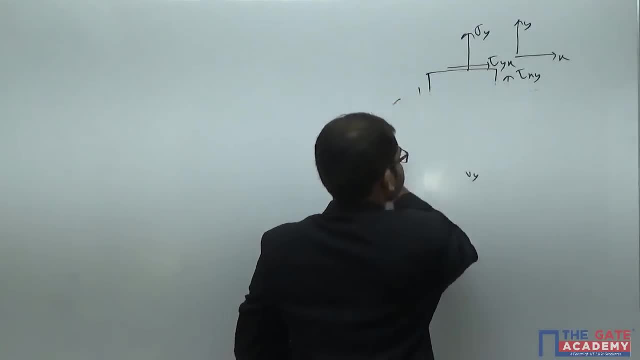 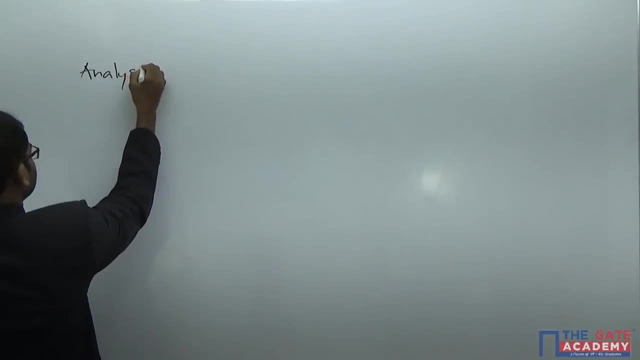 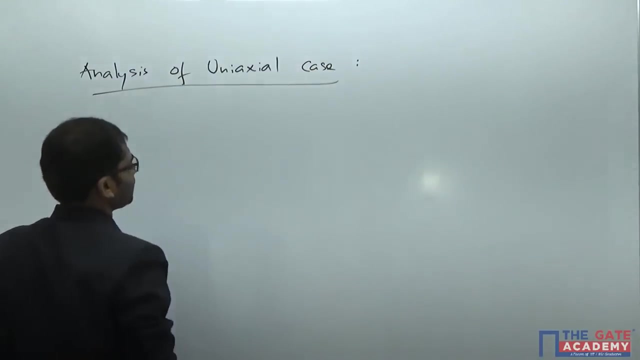 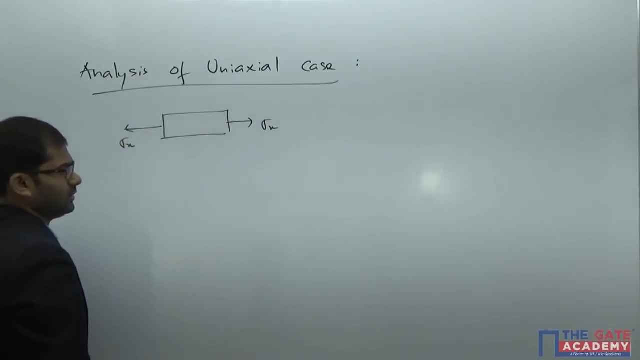 let's go with this uniaxial case. so i'm putting the title here. so it's very simple. here if you're mentally experiencing a tensile load in x direction, so it gives rest to transfer stress in acceleration here. so if you write down the stress tensor matrix, 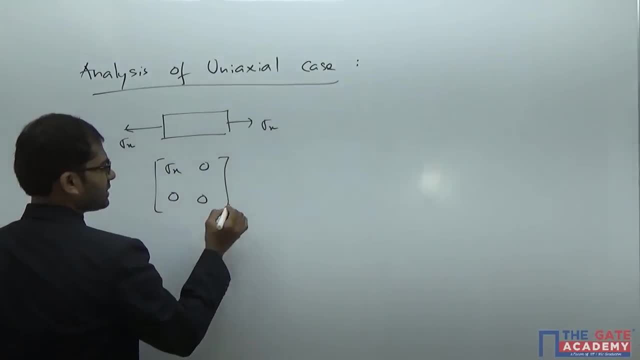 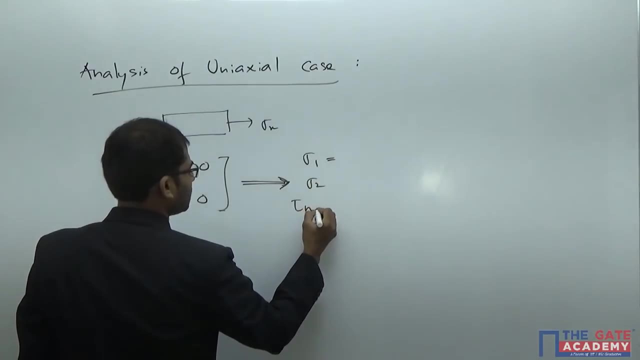 it will be simply sigma x, 0, 0 here. so for this case, if you find out, for this state of stress, if you find out, if you are finding out principal stresses, sigma 1, sigma 2 and also maximum shear stress. so sigma 1 will come as sigma x and sigma 2 will come as the stress of the stress, of the stress. 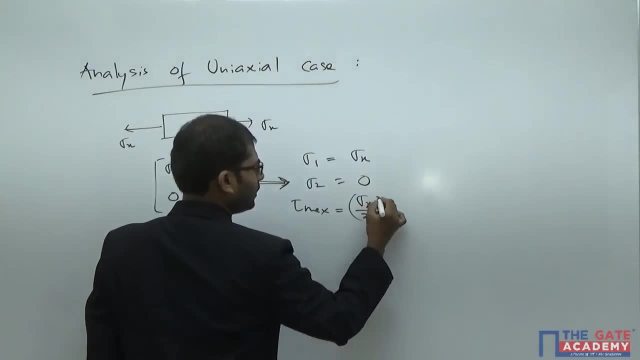 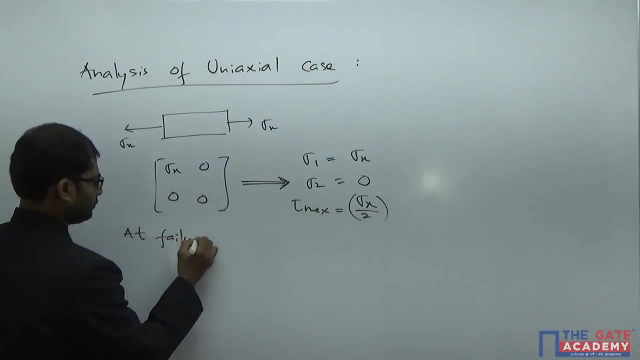 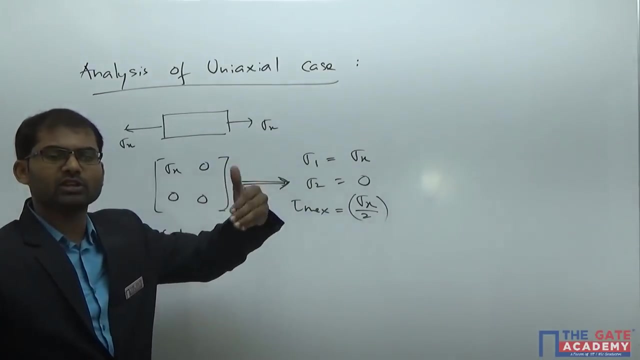 0 and sigma or tom1 matrix will come as sigma x by two. you can check the calculations of that. so now at the time of failure. so basically what happens is sigma x can be any value here, but the material can take sigma x value only up to yield point or ultimate point. it can't go beyond the strength. 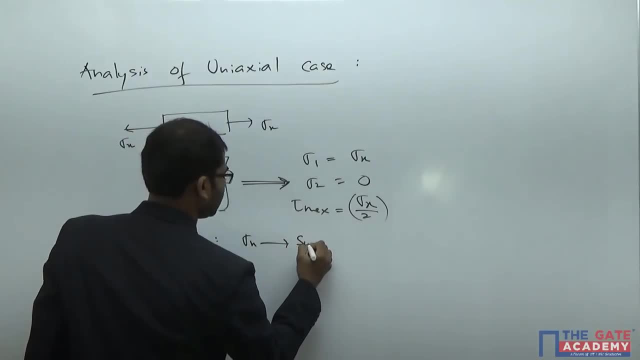 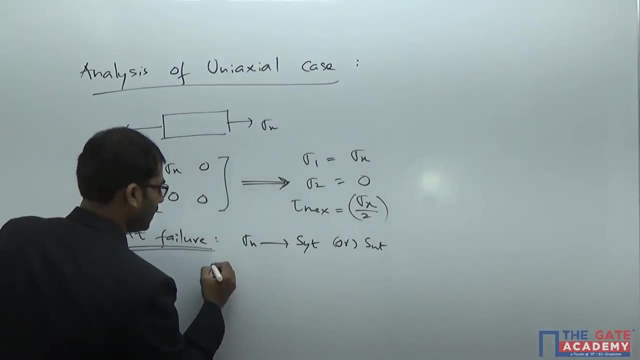 of the material. so at failure, this sigma x actually reaches, or tends to reach, the value of s y t or s u t value there. so as sigma is using s y t value, so at the time of subscribe of failure, principal stress, sigma1 is equal to sYt, sigma2 is equal to 0 and 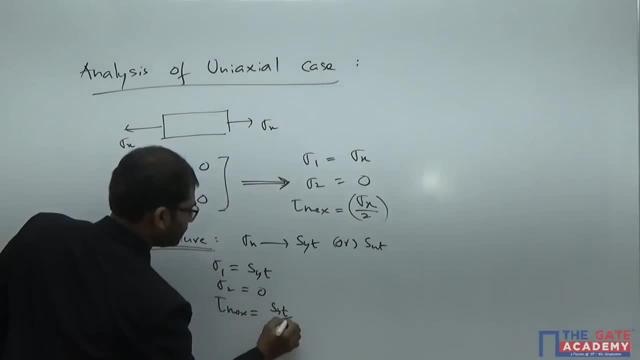 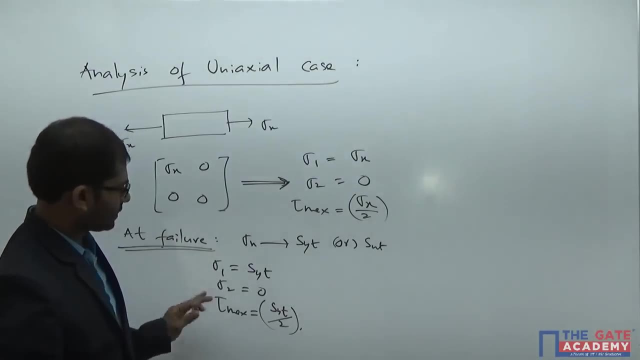 tau max value is equal to sYt by 2. You will be getting the value like this: If it is a brittle material, we will be having sUT sUT values here, This thing here. So you got all these parameters here Now, along with this uniaxial case. we should do the. 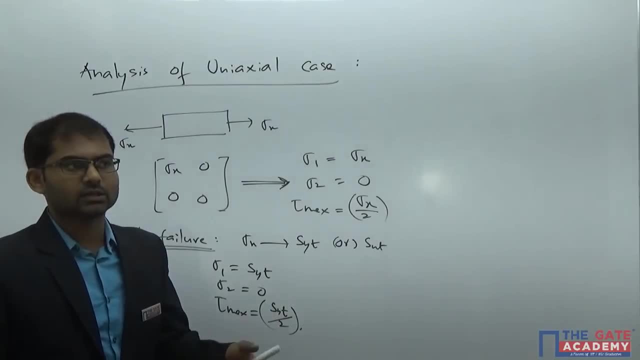 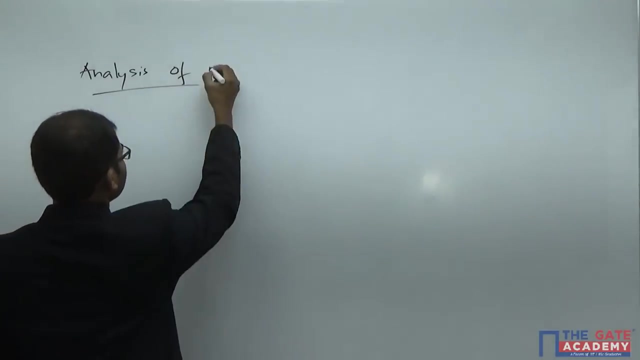 analysis of pure shear case also so that we can see the authenticity of the each and every theory of failure in an experimental way, So which you will understand very thoroughly later. So we are going with analysis of pure shear case. Analysis of pure shear case. So pure shear case means that loading 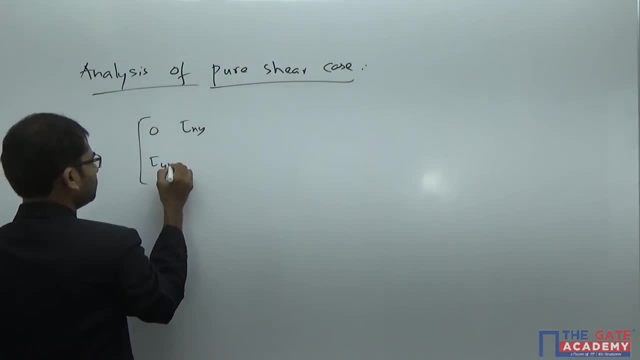 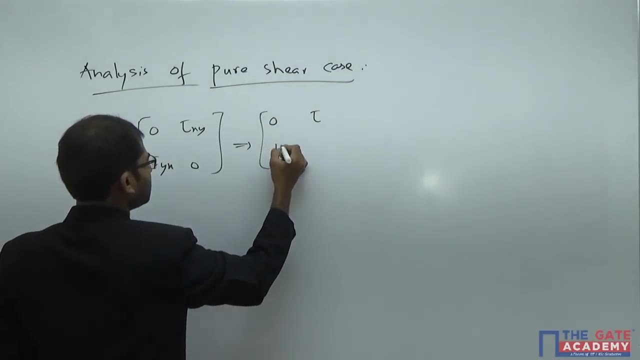 condition will be giving rise to only shear stresses: 0, tau xy, tau yx and 0 here, and where the parameters tau xy, tau x, both are same, So I will denote it by tau itself. So for this loading case, if you are, 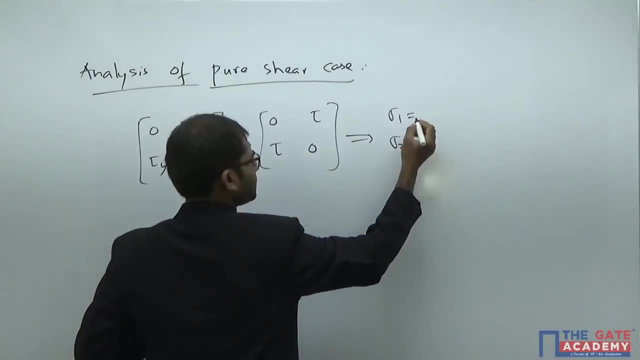 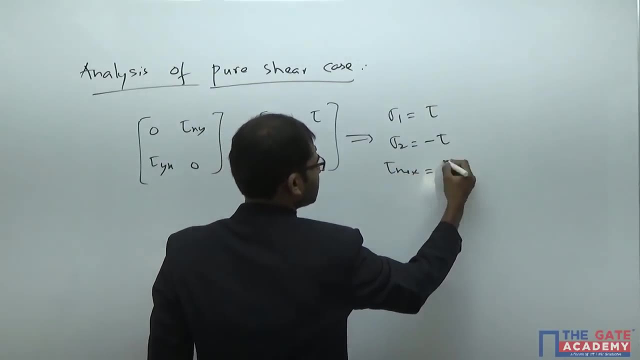 finding or principal stresses: sigma1 is equal to, sigma1 is equal to tau, sigma2 is equal to minus tau and you will be getting tau max value as tau itself. And this material also cannot take stress more than the strength of the material, in this loading case also. 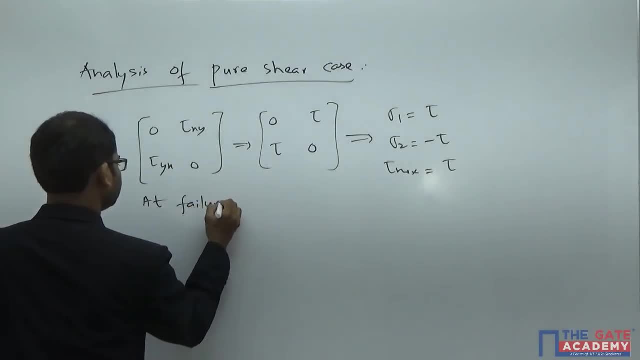 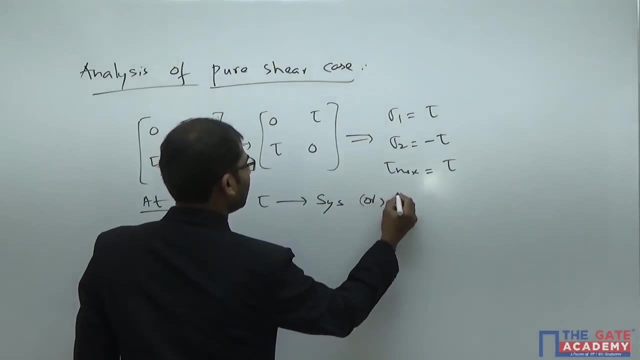 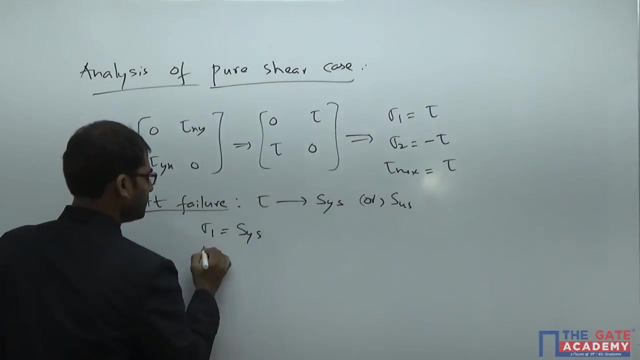 So, at failure, this tau value reaches sY. tau value reaches sYs or sUS. So here is the stress in shear, ultimate stress in shear. So this is the stress in shear. So your principal stress: sigma1 is equal to sYs, sigma2 is equal to minus sYs and tau max value. 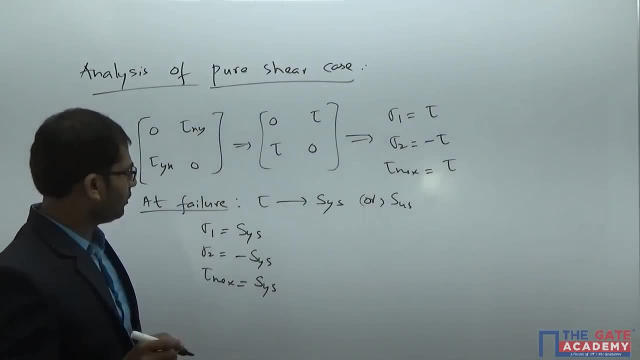 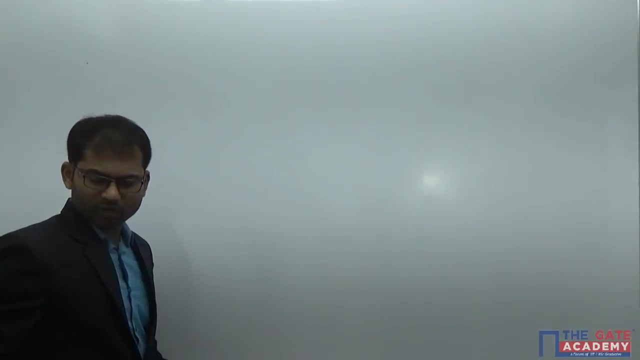 is equal to sYs itself. So if it is a preliminary, we will be having sUS minus sUS and sUS value. Now, before going into the first theory of failure or understanding the first theory of failure, we should have knowledge of assumptions we are going to take, or main, or important. 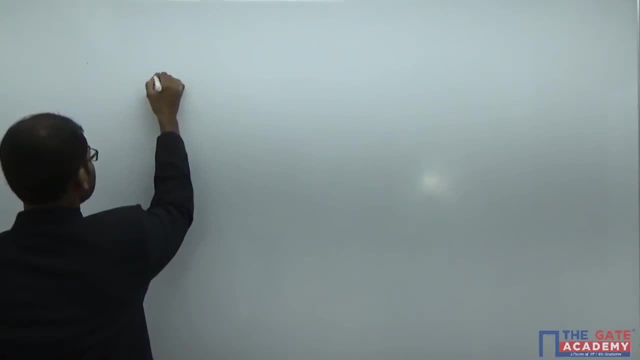 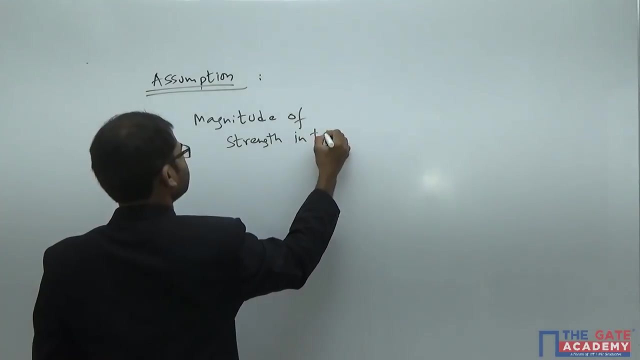 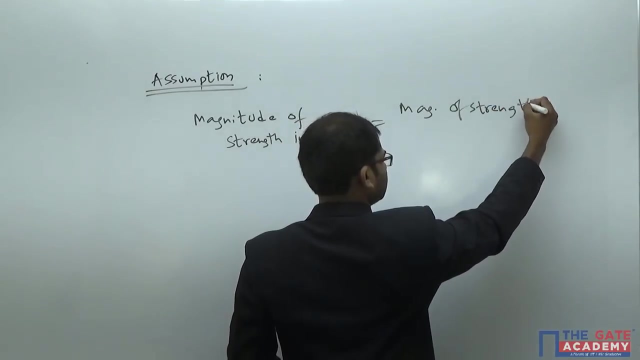 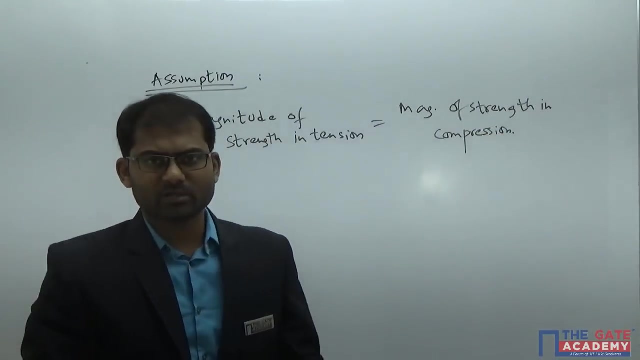 assumptions we are going to take for each and every theory of failure. So assumption here is: so we take the magnitude of strength of the particular material in tension is equal to magnitude of strength in compression, Because generally what happens is ductile materials. 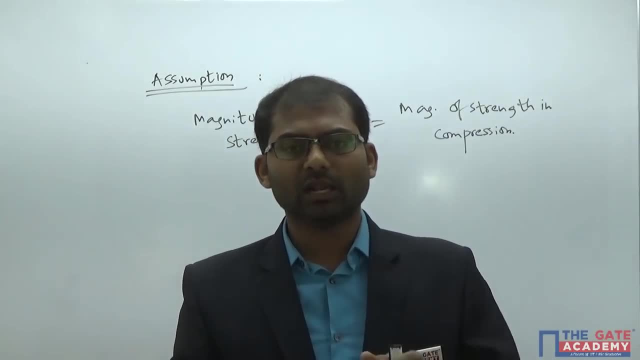 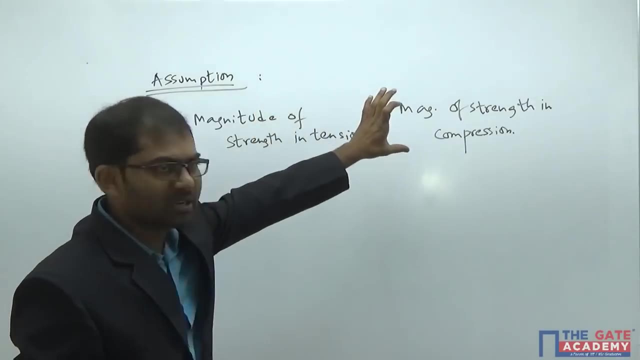 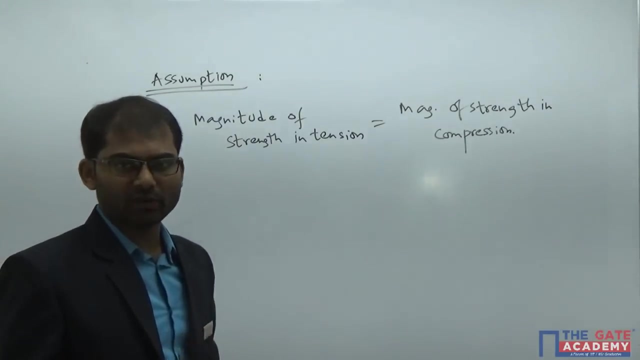 are in general stronger in tension and weaker in compression. So the left parameter is higher and right parameter is lesser. for ductile materials and for building materials it is reverse: they are stronger in compression and weaker in tension. So we don't go with the inequality in the study. 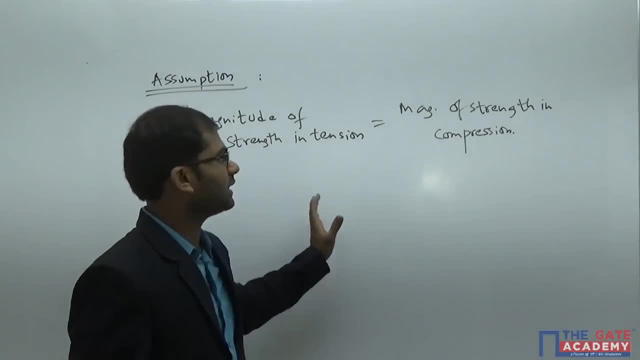 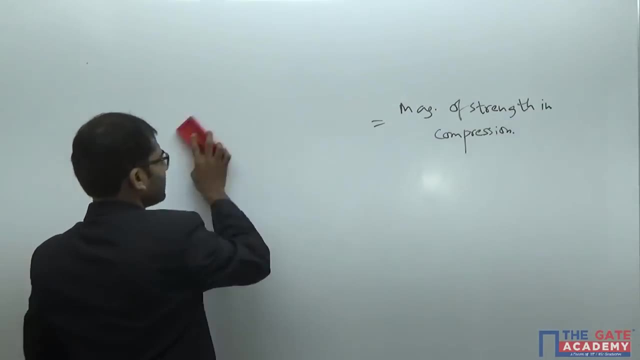 of theories of failure. So we take the assumption that magnitude of strength in tension is equal to magnitude of strength in compression. this is the thing which you are going to take here. Now let us go with the first theory of failure here: the maximum principal stress theory. 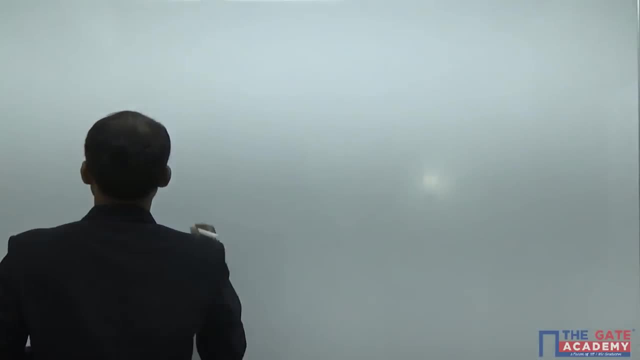 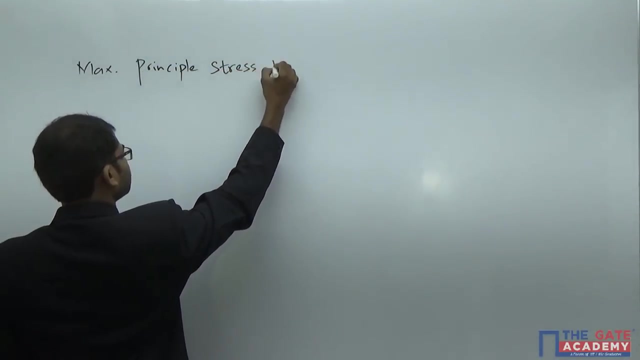 So from that we will understand how to deal with each and every theory of failure. So I am going with maximum principle, stress theory here. So it is a very simple theory here. So in fact every theory of failure is very simple. 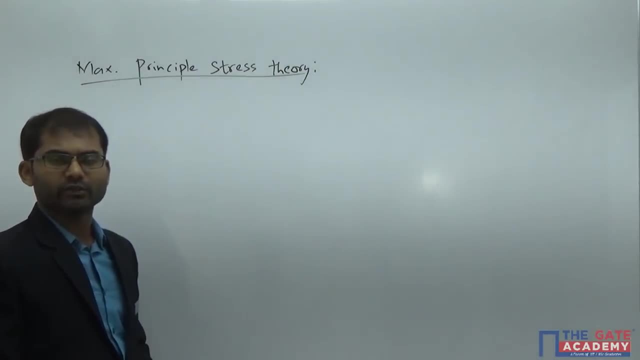 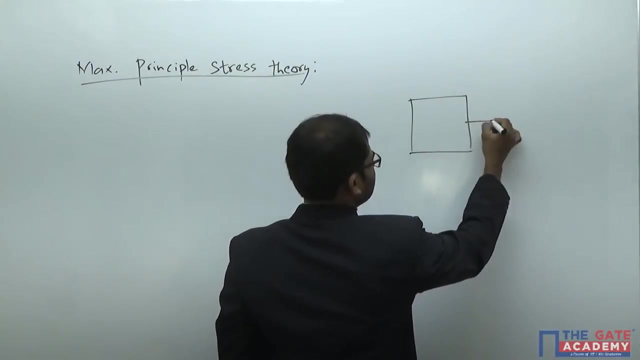 After completing of understanding these two theories of failure, we will come into the particular stage. So I said that, what is the basic principle? So we take the maximum principle stress for our combination loading case here. So we have sigma x, we have sigma y, and also tau x y and tau y x. 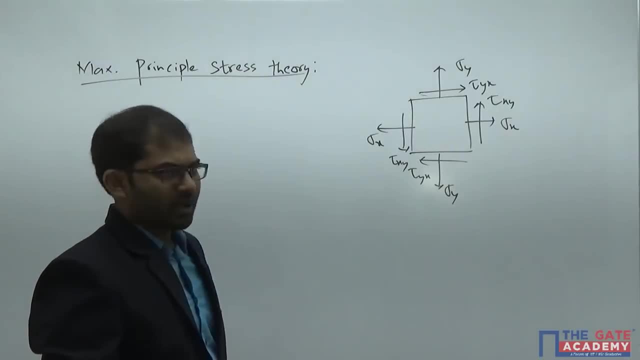 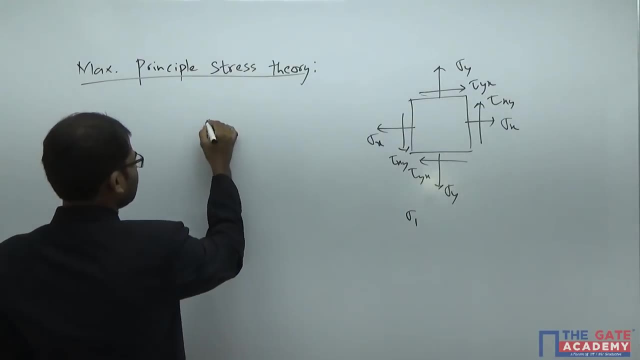 So we got these values here. So maximum principle stress is same. So for this one we will get the value of maximum principle stress, sigma 1.. We will compare with the maximum principle stress of the same material in uniaxial loading case. 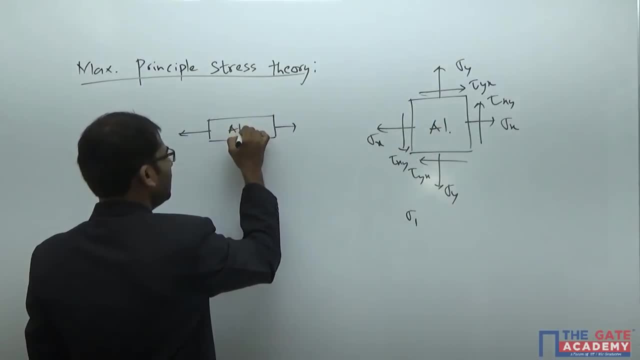 So both the metals must be same. If it is aluminium, it should be aluminium. If it is copper, it should be copper. The other way it does not make any sense. So we find out sigma 1 for uniaxial loading case at failure. 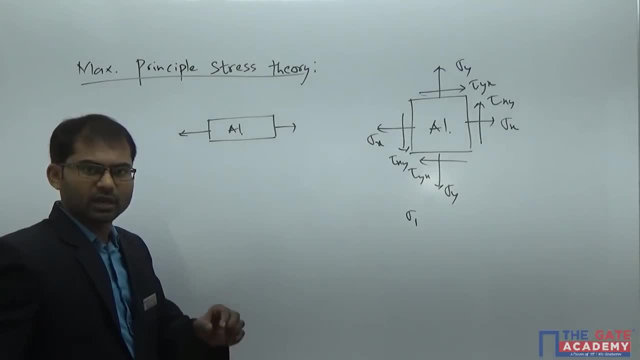 So sigma 1 for uniaxial loading case at failure. if you turn your base and check it, you will be finding out that sigma 1 is sigma x in a general loading case and sigma x value will reach the time of failure as s y t value there. 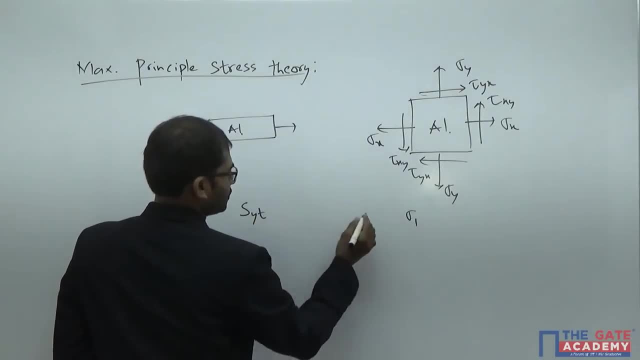 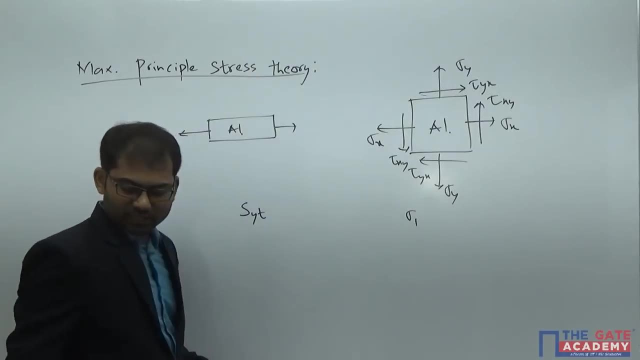 So sigma 1.. So sigma 1 is equal to s y t. So here it is s y t here. So this sigma 1 should be less than s y t for failure not to occur. If we need to go with the critical condition, then we need to take this as equal to here. 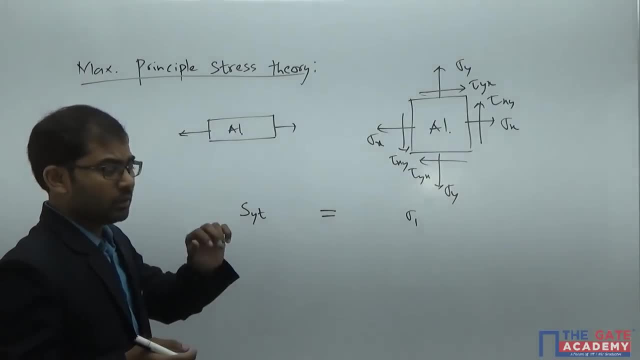 We will take this one as equal to here. Now, sometimes- sorry, sometimes- instead of designing the material with respect to failure, stress or the strength of the material, we will be designing with respect to allowable stress. But you know, allowable stress is equal to s y t. 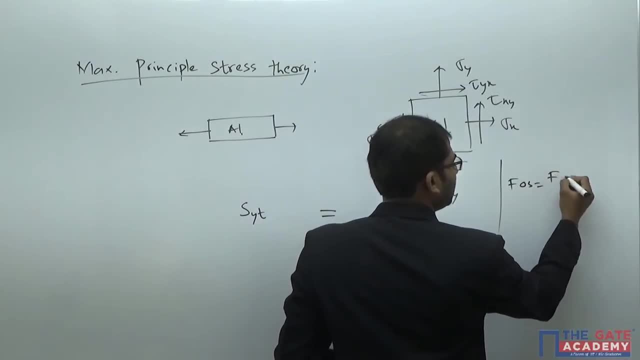 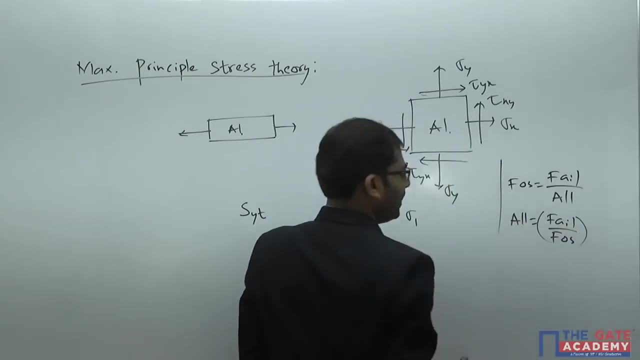 So that is equal to- or we have: factor of safety is equal to failure stress by allowable stress. That means allowable stress is equal to failure stress by factor of safety. So if you are taking factor of safety instead of s y t value, which is nothing but failure stress, 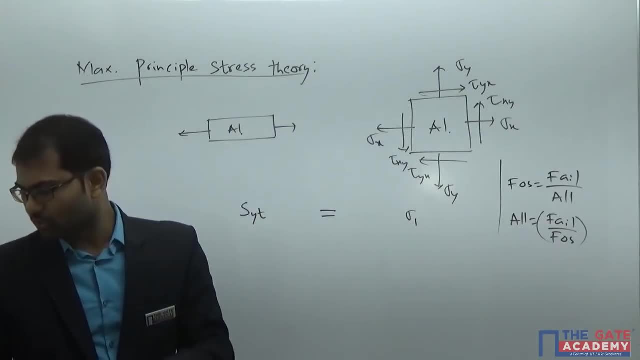 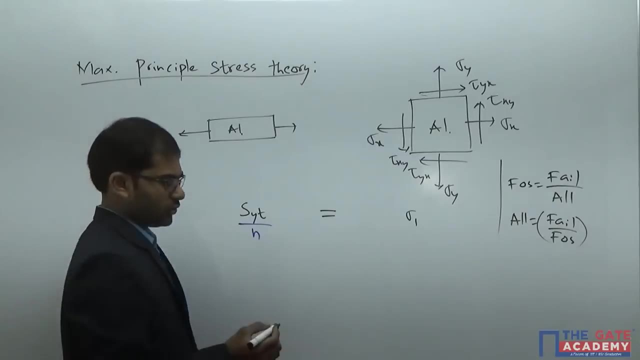 I will be putting allowable stress with this failure, stress by factor of safety. So you will be having n in the denominator on the left side if you are taking the factor of safety value here. So this is the equation here. So you got the equation number 1 here. 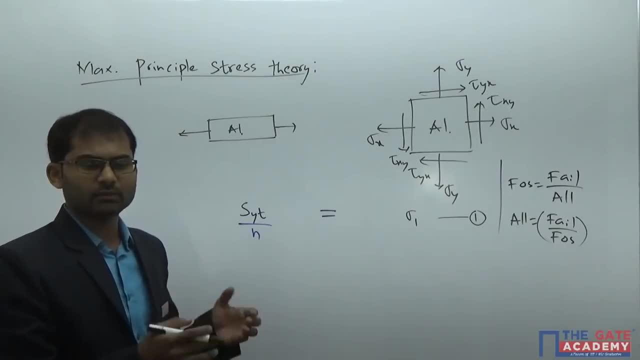 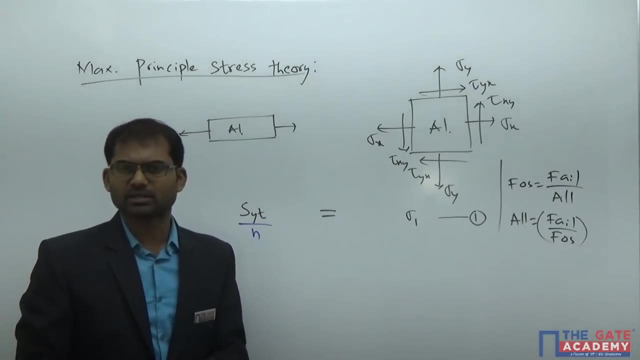 So remember, every theory of failure will be having: 2. equations and a diagram that will help you to solve any question from questions, of any question of gate level or even IES level or basic mechanical engineering papers levels there in most of the complete examinations here. so now this. 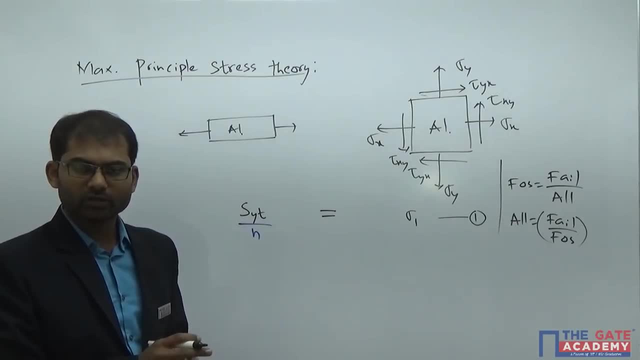 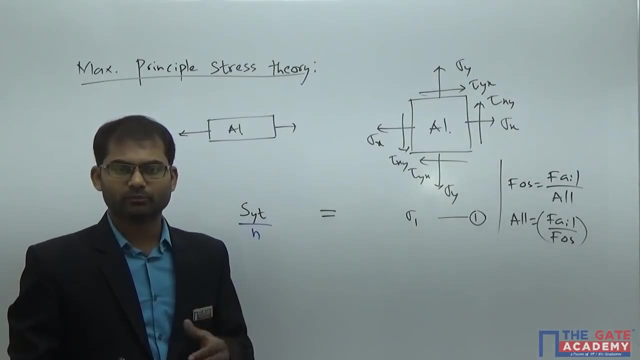 theory is given like this, but we don't know how authentic it is. how authentic is the theory of failure here? so we should, practical way or in a by experiment, we should decide whether it is true or not, or it is valid for only number of materials or which type of materials. basically. so to do that, what? 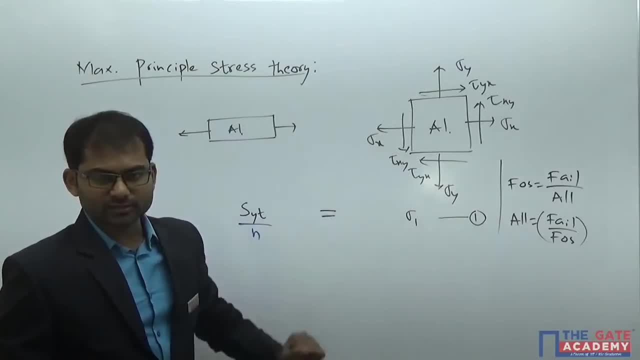 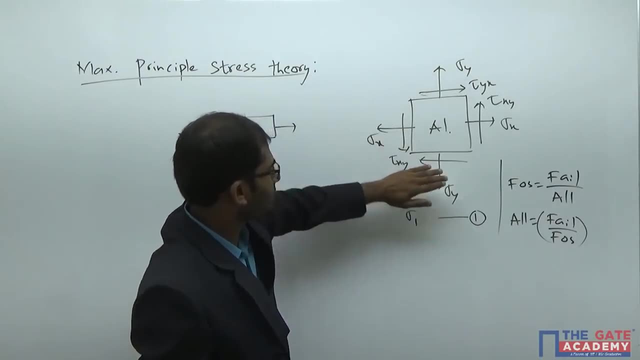 we're going to do is. I'm going to take an example of this particular loading case. I'm taking an example where Sigma X is not there, Sigma Y is not there. Sigma X is not there, Sigma Y is not there. I'm taking example: if Sigma X, Sigma Y are. 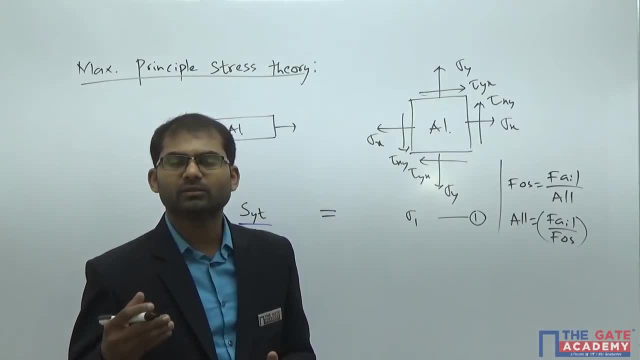 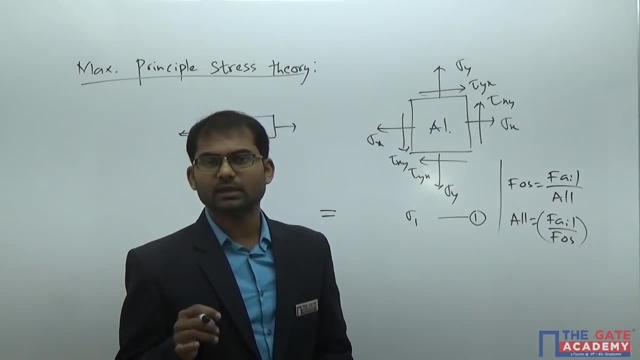 not there. only tau xy, tau yx are there. it's simply nothing but a pure shear case. I'm substituting Sigma one for pure shear case. Sigma one for pure shear case. E is given by tau. at the time of failure, this tau becomes s y s value. 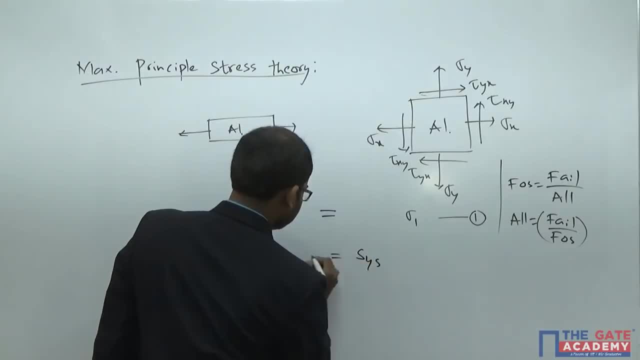 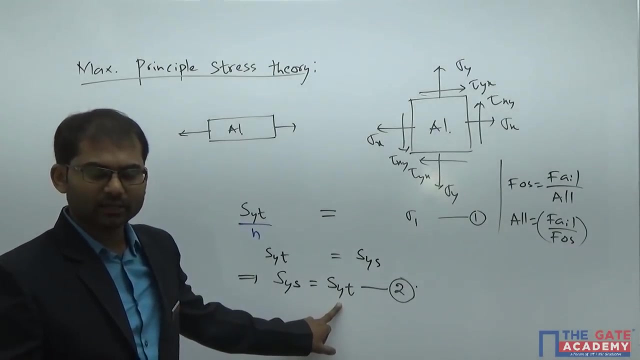 okay, so this becomes s y s, s y t. generally, this s y s is written on the left side, so this equation becomes: s y s is equal to s y t, the equation number two. so this is an experimental value. this is an experimental value here. I can say that. 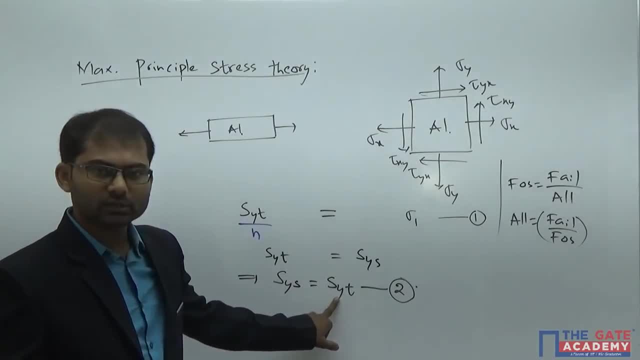 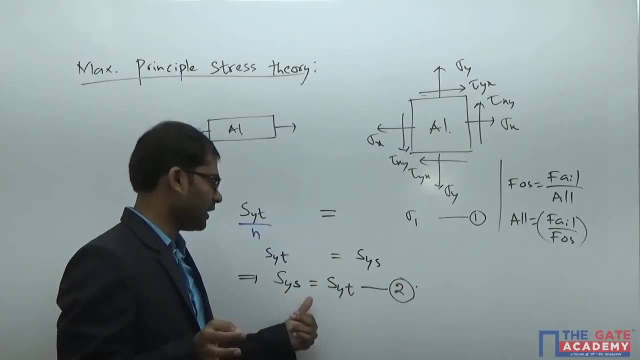 whatever the material is there, it is going with these which actually satisfy this relation. that means I take some material. I take some material, do the tensile testing and find out s y t value, and I'll take the same material, do the shear testing. I'll find out s y s value here. so if those 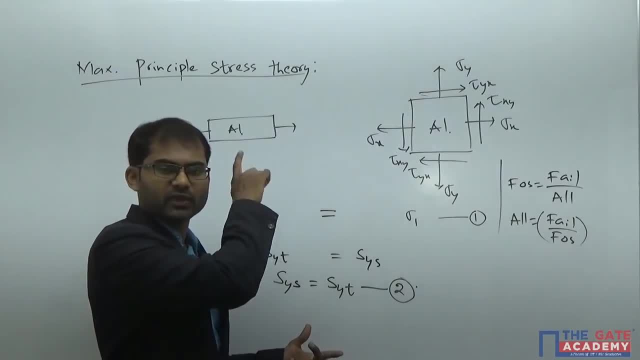 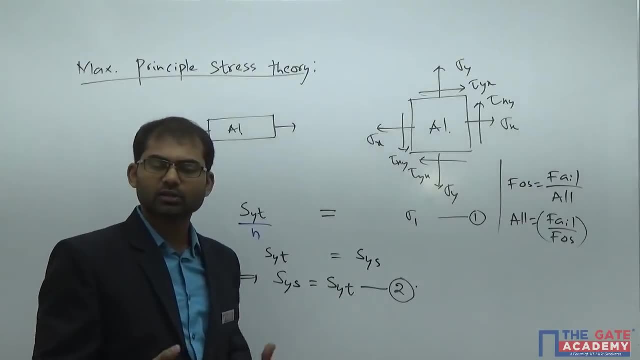 values are coming as equal, then I can say that this theory of failure is valid only for the material, or for the materials which are actually satisfied in the relation. if the material is giving you this value is a half of this value, then it's not going to be satisfied. they are so for experimented, observed. 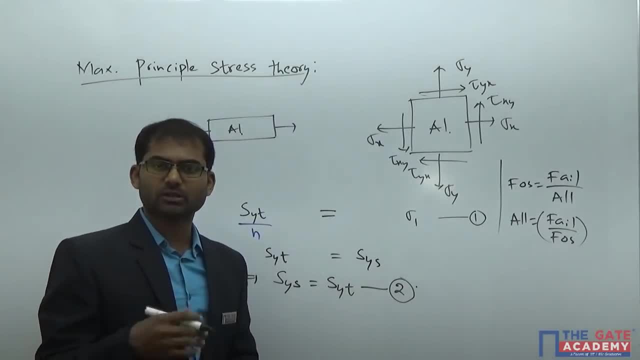 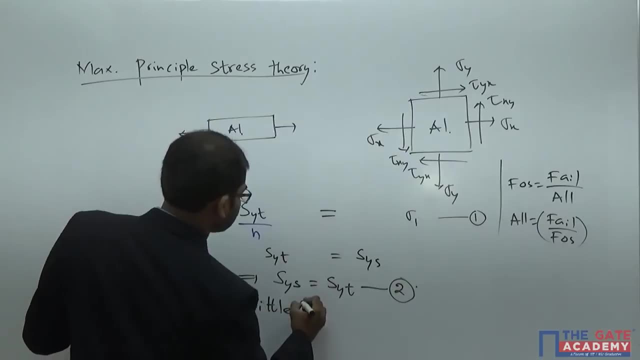 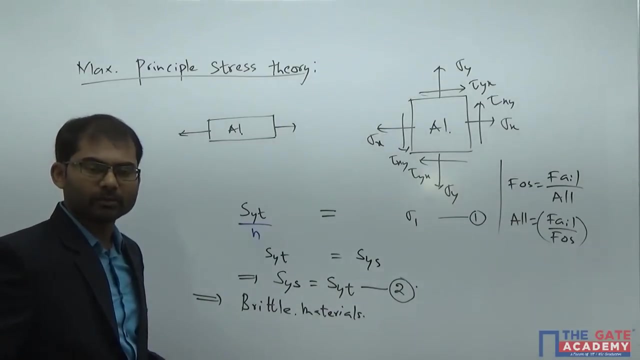 that out of the different, different, well types of measures which are present on, they understood that this equation is being satisfied by brittle materials. so there is to some sort of brittle materials. so this theory of failure is valued for. this theory of failure is actually valid for some sort of brittle materials, but because of 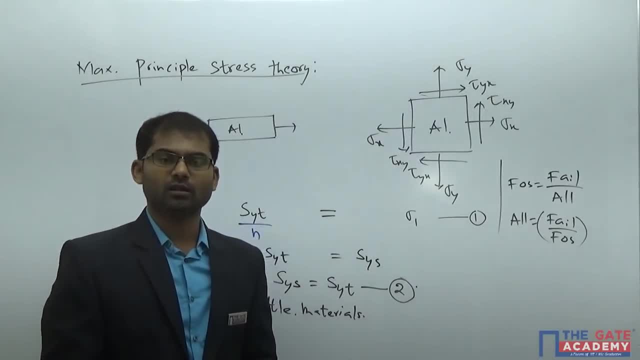 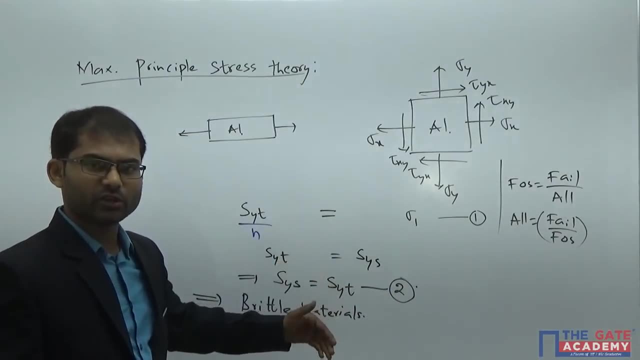 simplicity, this theory of failure is taken as valid for all the types of all the types of brittle materials there. so we are turning these two equations here. so if you apply the same concept in every theory of failure, you're going to derive equation number one, equation number two here. so 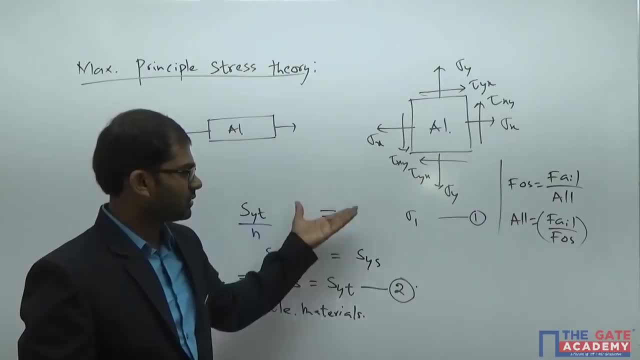 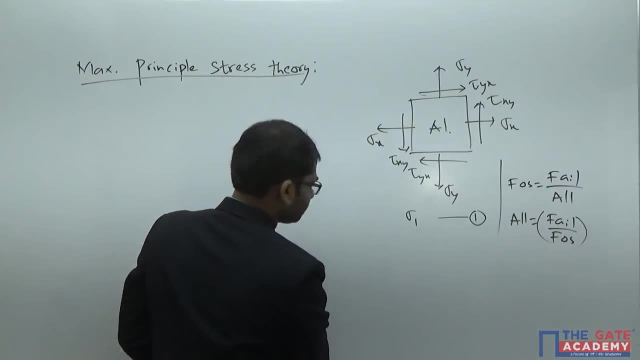 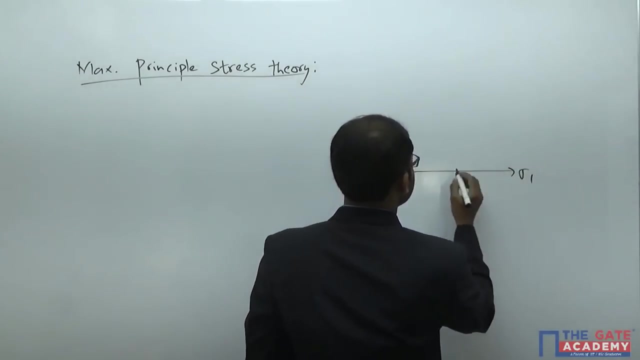 we need to know the reason of safety also. so i will give you the derivation of reason of safety for this theory of failure also here. so i'm drawing the reason of safety now. reason of safety is nothing, but we're going to draw a curve on a cartesinal system which is having sigma 1 axis. 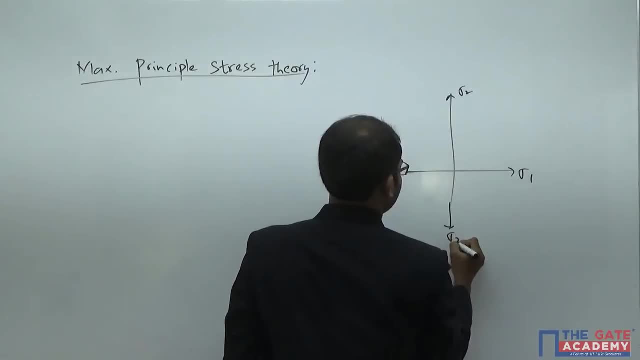 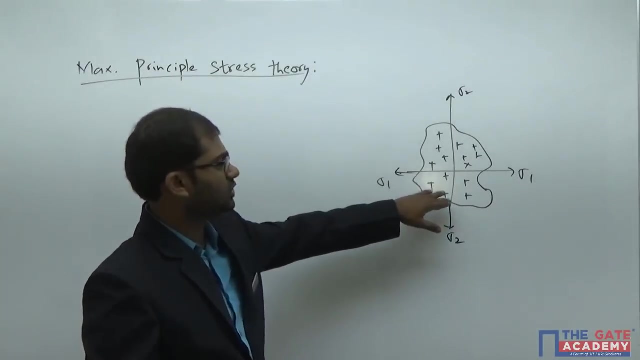 as x axis and sigma 2 as y axis here. so we'll find out the reason of safety here. so this reason of safety will be having plots of sigma 1, comma, sigma 2 here. so this sigma 1, sigma 2 values will be inside the region like this. so if your sigma 1, sigma 2 coordinates are coming inside this region, 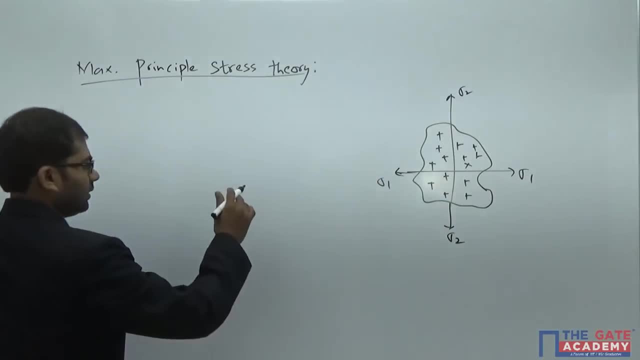 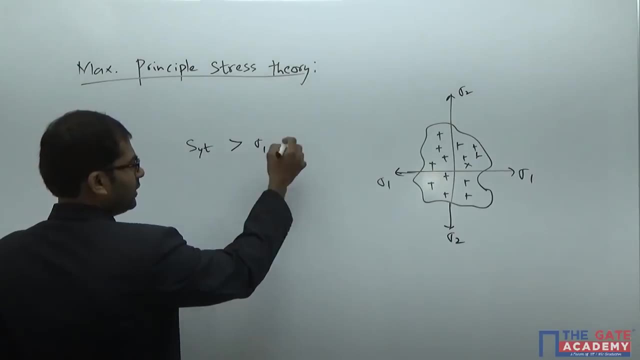 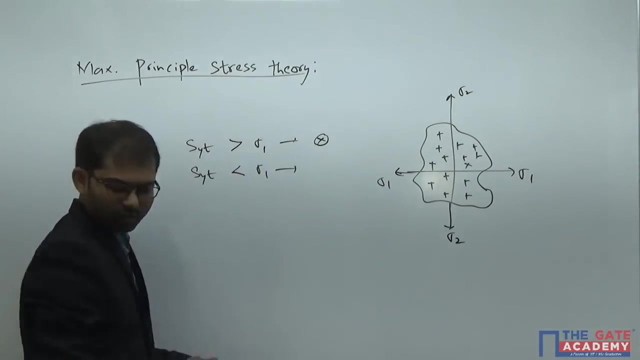 that means the you for that means the metal going to be safe. that means here s y t greater than sigma. this equation is satisfied. this inequality is satisfied here. okay, so this is divided by this point here, if you are having s y t is less than sigma 1. so these are all divided by other line. other points here. 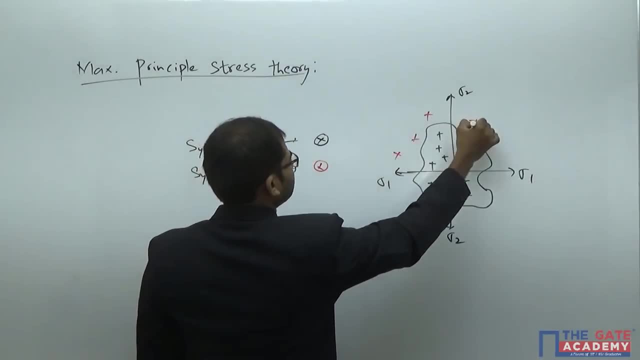 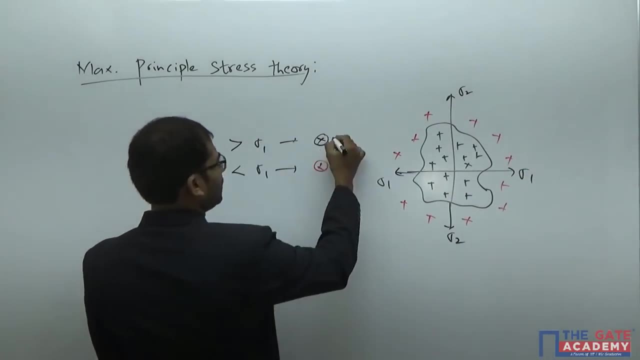 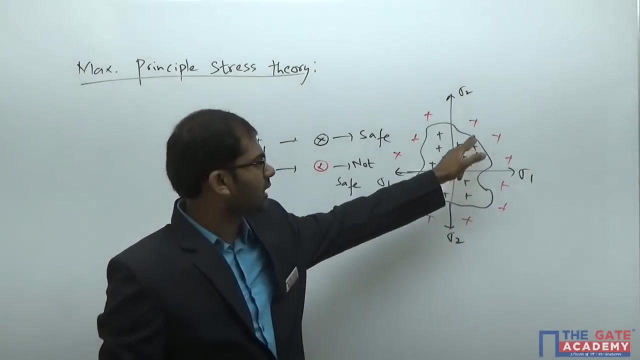 which i'm denoting it by that means it's not going to be safe here, so here it is safe and here it's not going to be safe, so this is safe conditions and these not safe conditions. so for every theory of failure, this region curve will be going on. 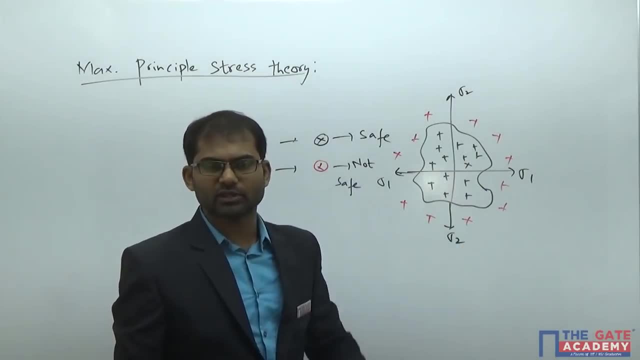 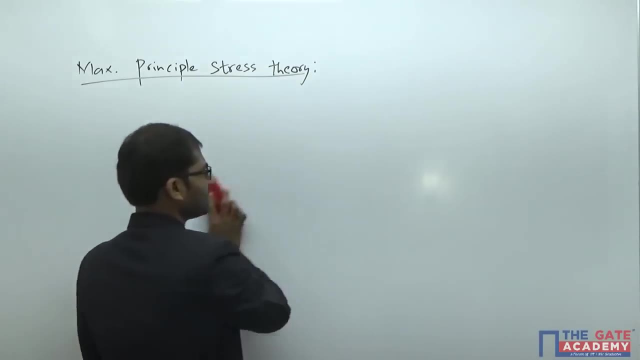 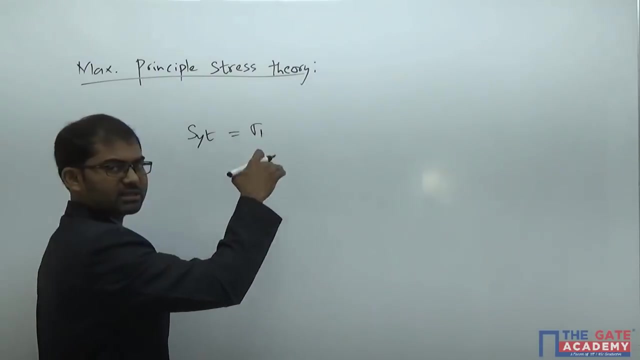 changing. the equation of the curve will be going on changing for each and every theory of failure here. i will try it for this theory of failure now. so our theory of failure is having equation number one, which is basically given as s y t is equal to sigma 1. so this is the condition if sigma 1 is. 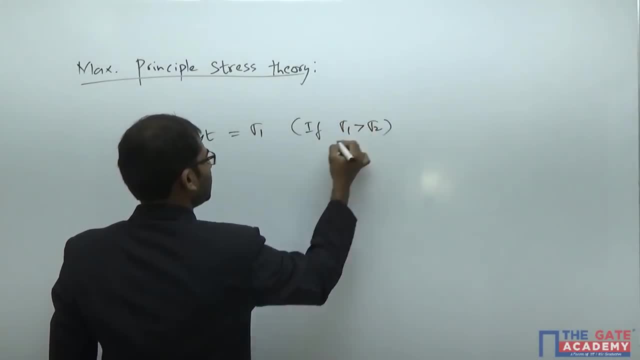 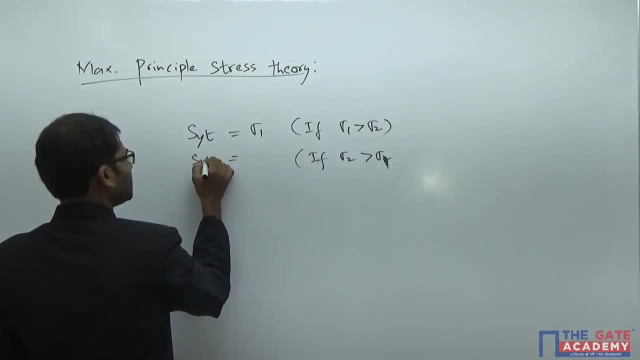 greater than sigma 2, if sigma 1 is greater than sigma 2. here, if your condition is: sigma 2 is greater than sigma 2, sigma 2 greater than sigma 1, then your equation will become: syt is equal to sigma 2. here now, if you take this 10 compressive loads, syc is equal to sigma 1, syc is equal to: 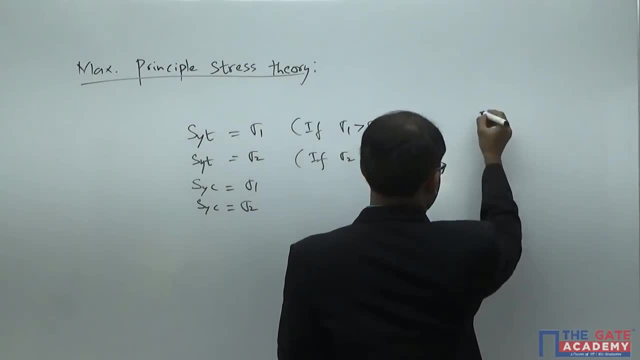 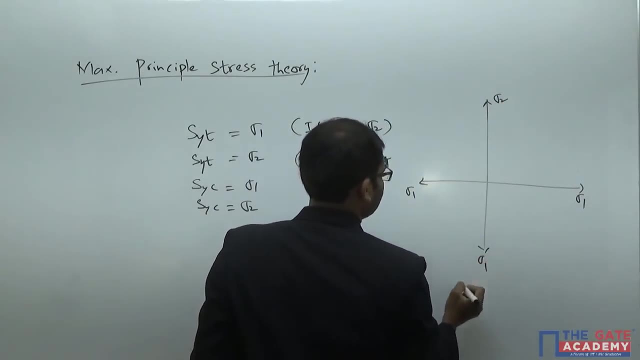 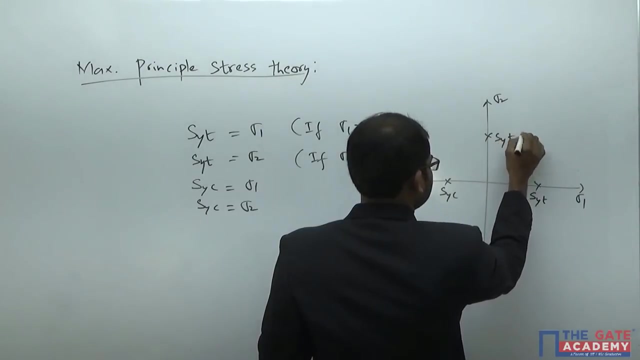 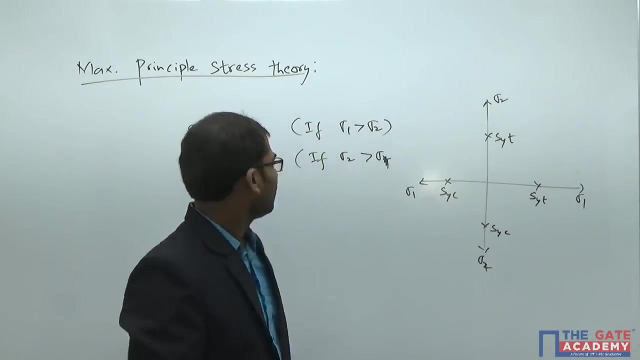 sigma 2. now you draw these four lines on a graph having sigma 1 and sigma 2, so you take this one as syt, syc, syt and syc values, because anyways you know magnitude of this syt and syc values here. now you draw these lines, first one i'm drawing here: syt is equal to sigma 1, syt is equal to: 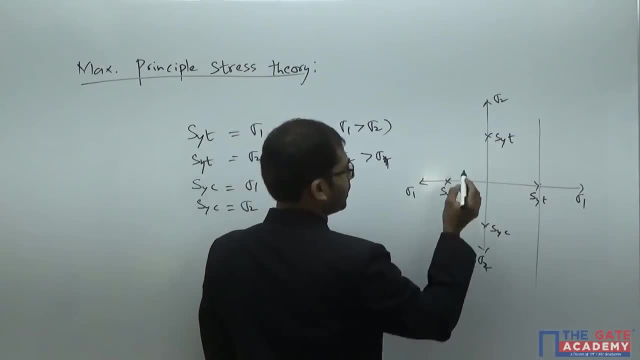 sigma 1 means this is a line, vertical line. syt is equal to sigma 2, syc is equal to sigma 1, syc is equal to sigma 2. so in this one you're gonna get sigma 1, sigma 2 values inside this region like this: 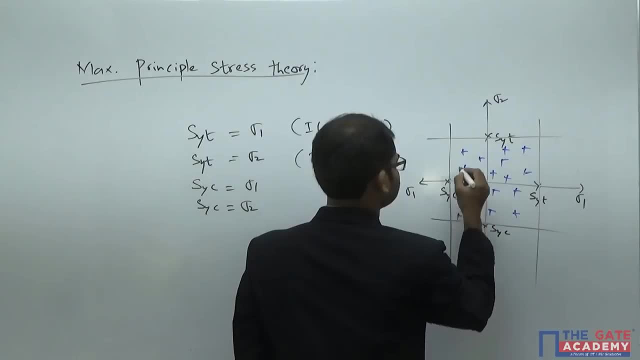 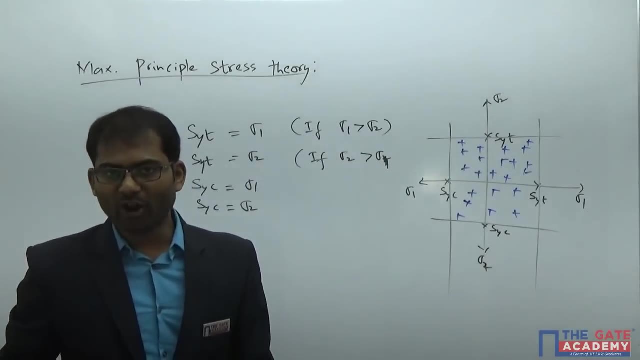 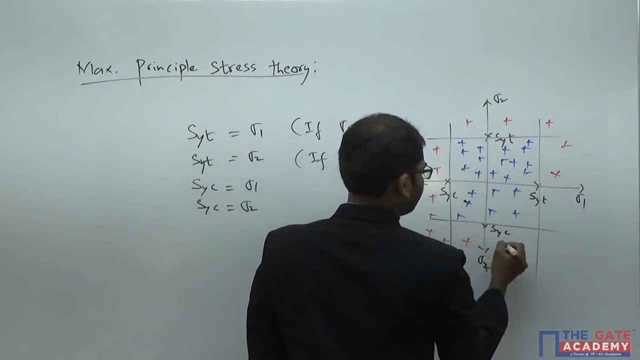 so these values are coming inside this region- this blue points- then the middle going to be safe. if they're coming outside this region, the middle not going to be safe. so you don't need to worry regarding the proof of this particular regional safety diagram here. but if you're just remembering, 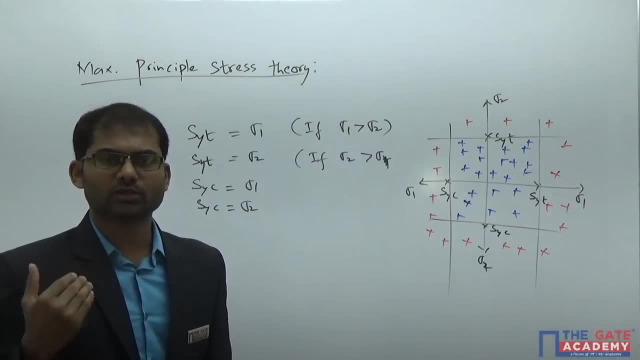 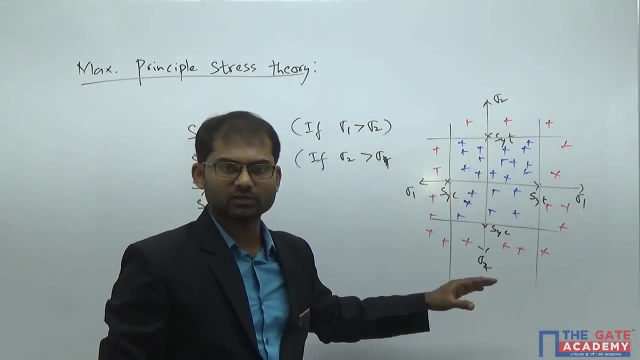 the shape of the diagram, at least you'd be able to solve all these questions from previous GATE papers. so if you're preparing by Sethgate, just remember how the shape of the diagram is coming. so what? the shape of the diagram, basically. so it's square here you just have. 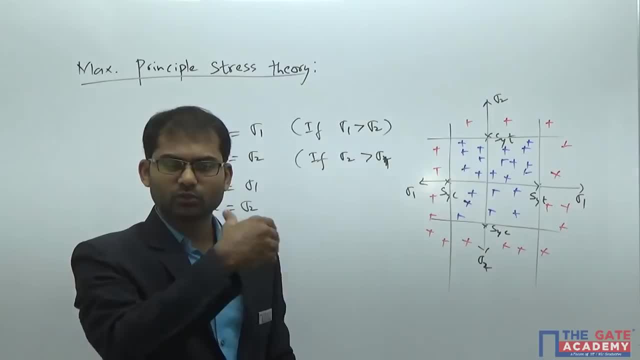 to keep this right here. now i'm applying the same concept to evaluate the expression or equations and diagrams for Maxwell shear stress snake. so the same way we do it for all the theories of failure also, i'm doing it for chequa. so of a, doing it for maximum shear stress theory now. So let us go with the maximum shear stress. 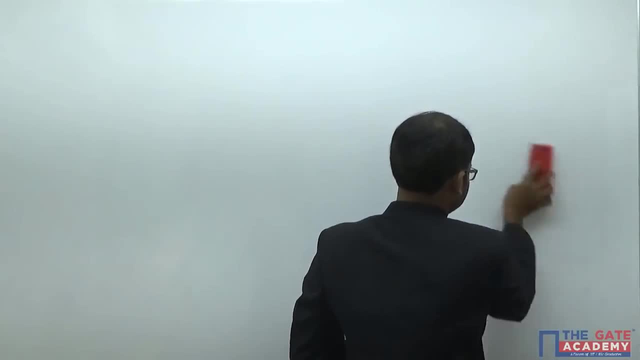 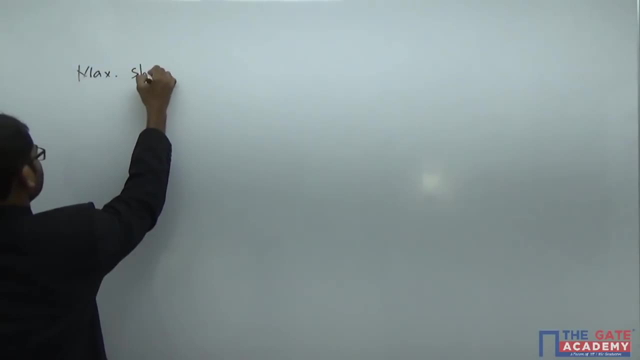 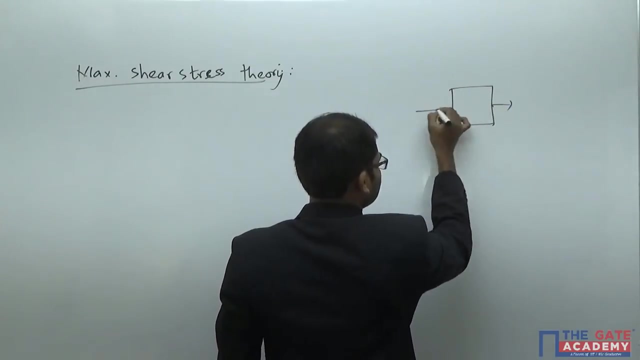 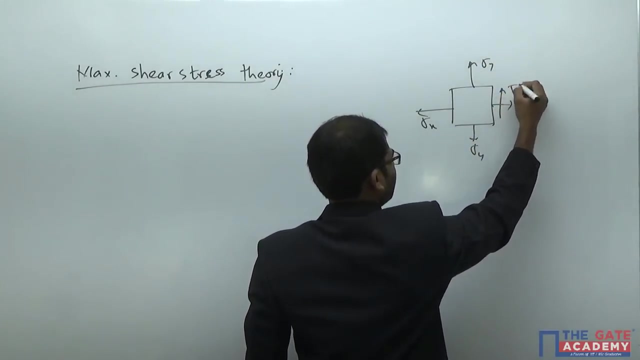 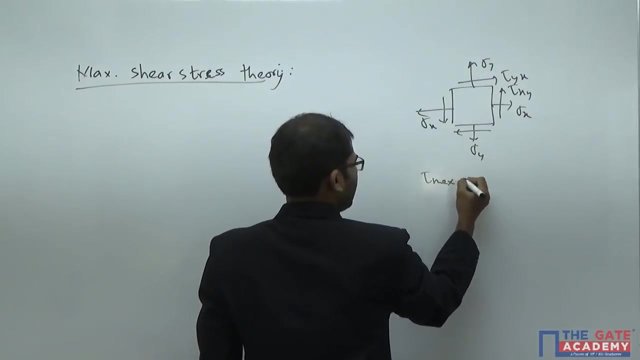 theory. So for a maximum shear stress theory, it says that. so for our loading case. so for our loading case, we need to get the value of maximum shear stress. sigma x, sigma x, sigma y, This is tau x- y. So let us get the value of tau max here. Tau max is equal. 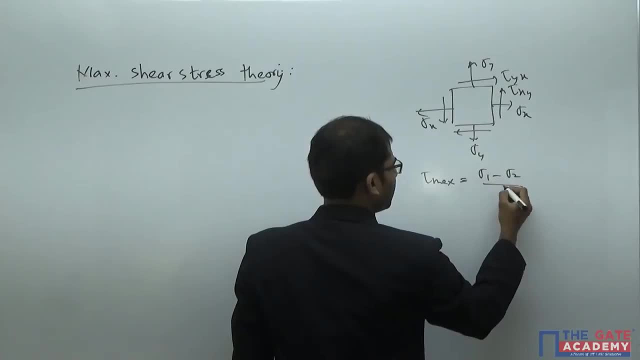 to given by. we can write down as tau max as sigma 1 minus sigma 2 by 2.. For 2D state of stress, I am first of all denoting it by 2D state here, where loads are acting in two. 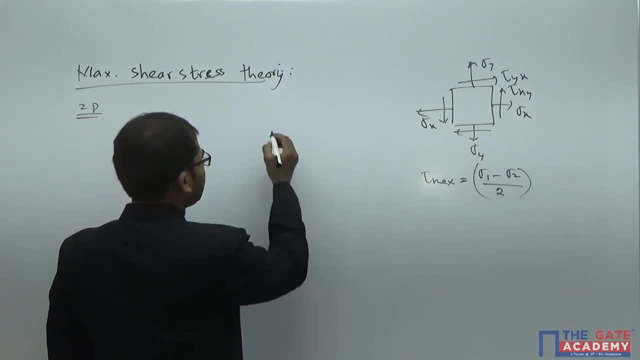 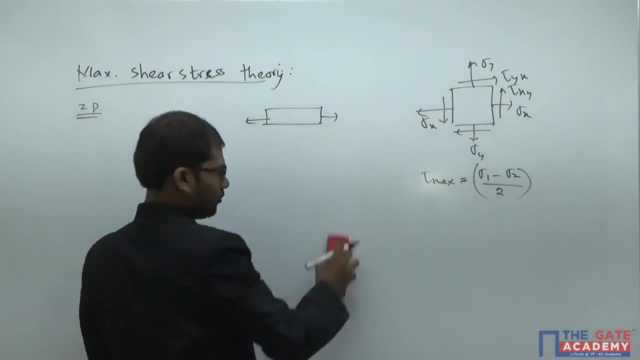 directions. Tau max equals sigma 1 minus sigma 2 by 2.. So we have to get the value of maximum shear stress theory. So let us compare it with the same material in uniaxial loading case. So in uniaxial loading case you will be having tau max value at the time of failure. 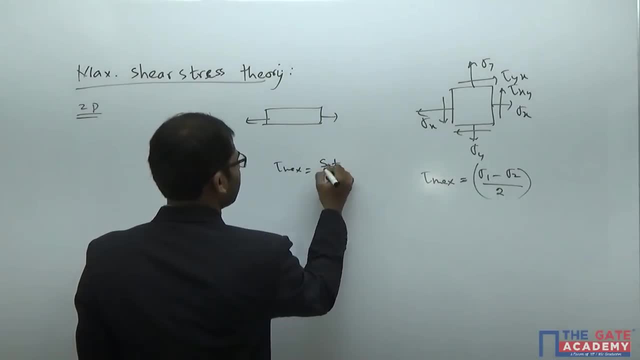 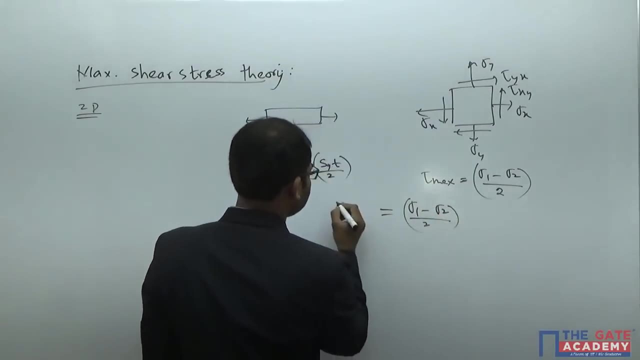 as so here tau max is equal to s y t by 2.. So for your material to fail, your sigma 1 minus sigma 2 by 2 should at least become s y t by 2.. Once this value reaches this value, 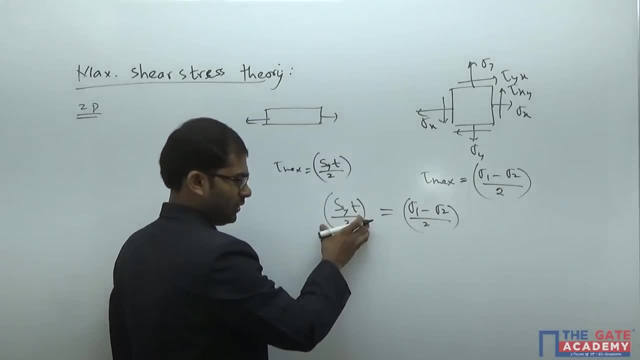 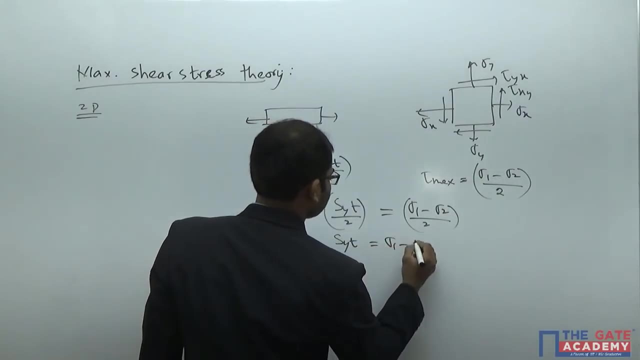 failure will happen. Once this value is lesser than this value, the material is going to be safe. So if it is more than this value, automatically it is not going to be safe. here, If you simplify this relation, you are going to get it as s y t is equal to sigma 1 minus. 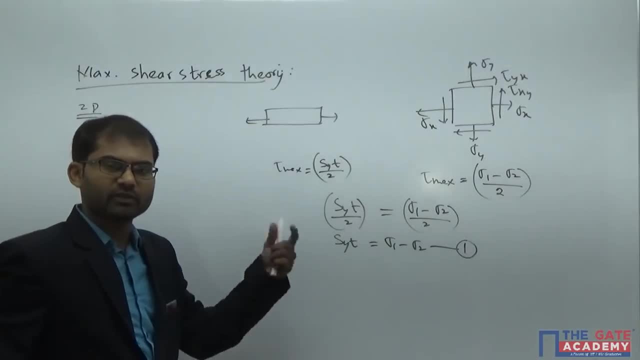 sigma 2.. This is equation number 1.. That is like we got equation number 1 in the previous theory of failure. We are getting equation number 1 in this case. here s y t is equal to sigma 1 minus sigma 2.. And if you are going with factor of safety, you will be having 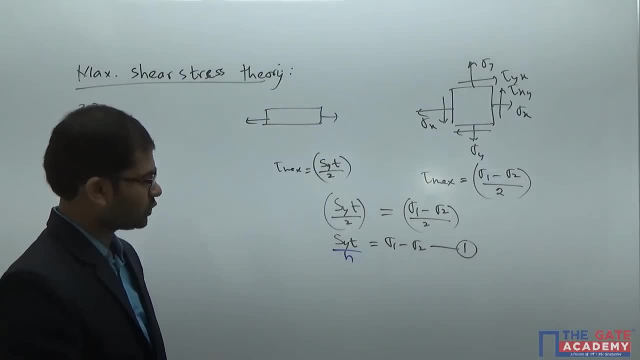 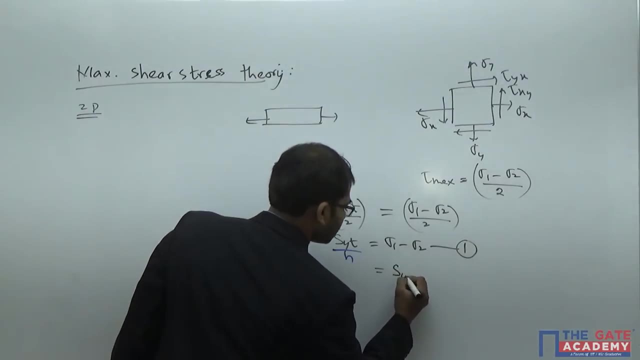 n here. Now to derive equation number 2, we have to substitute sigma 1 sigma 2 in terms of pure shear case. So sigma 1, sigma 2 in pure shear case is nothing but sigma 1 is s y s and sigma 2 is minus. s y s is equal to s y t. 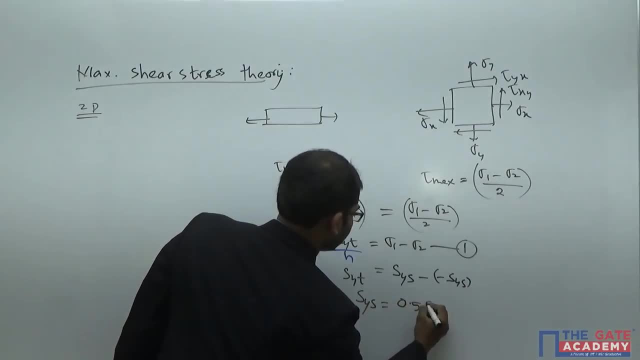 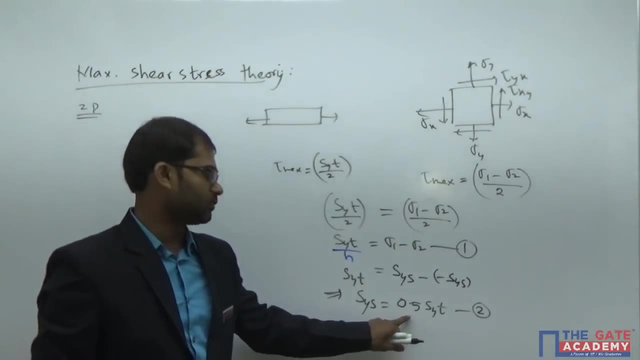 So if you simplify this, this will become s y s is equal to 0.5 s y t. This is equation number 2.. In the earlier theory of failure we got s y s is equal to s y t, but here it. 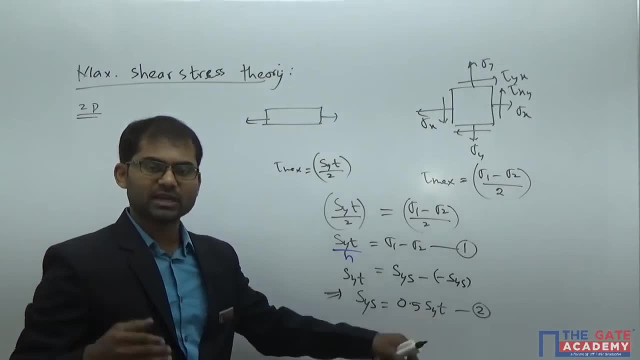 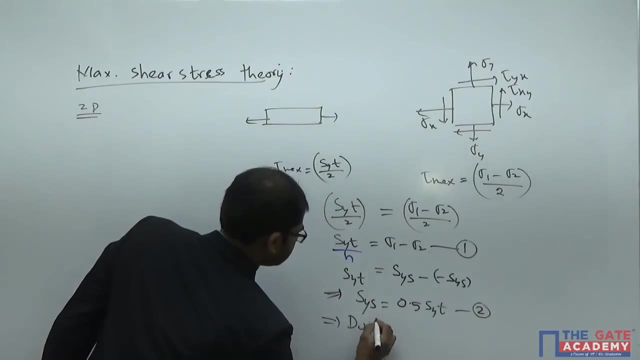 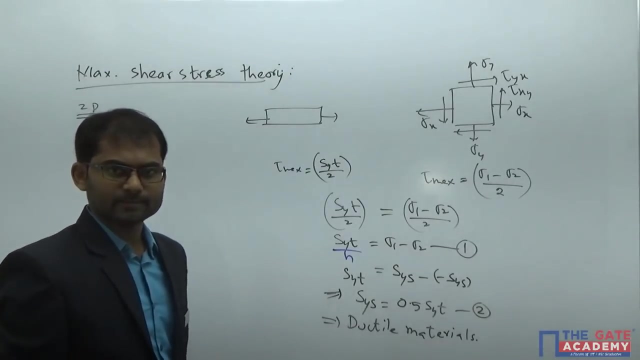 is 0.5 s y t here, And this equation is actually satisfied by the ductile materials only, So it is valid for only ductile materials. So it is like this: We will have to derive equation number 1, equation number 2 in this way and we have 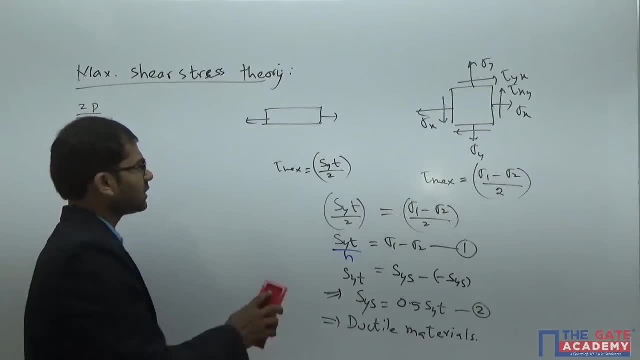 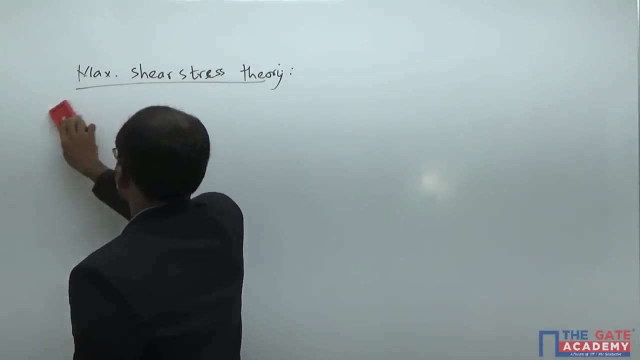 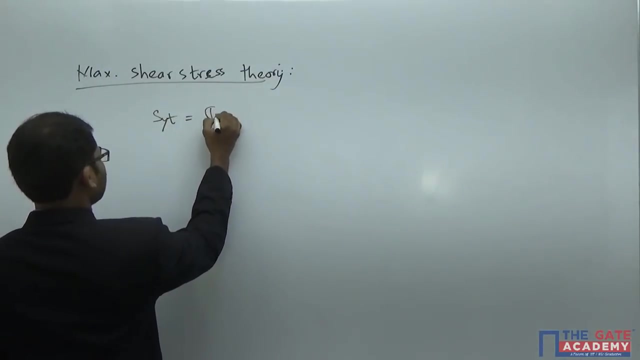 to do the calculation Now if you are going with the region of safety. So, region of safety, to draw the region of safety we need equation number 1.. s y t is equal to sigma 1 minus sigma 2.. Anyways, we are drawing the graph between only sigma 1 and sigma 2.. We are not. 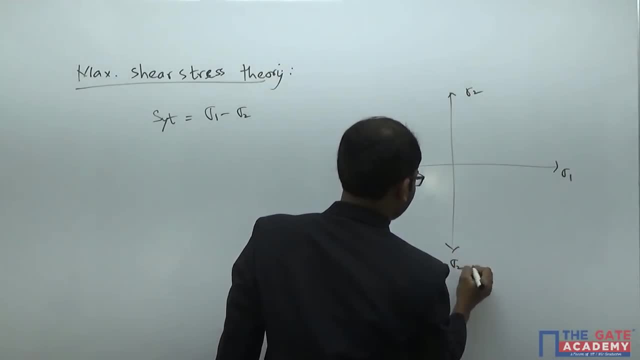 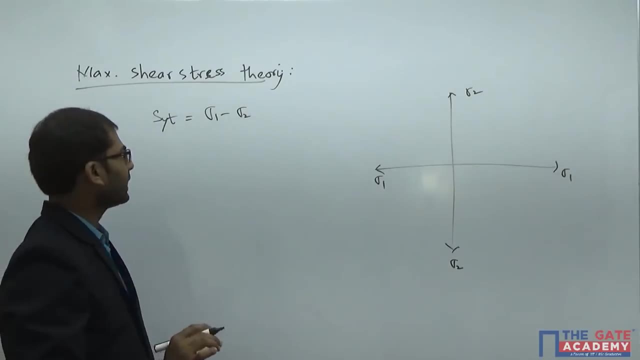 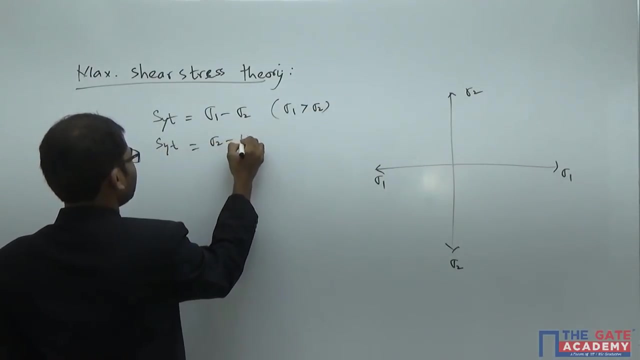 concerned regarding. We are not concerned regarding this particular sigma 3.. So we are concerned regarding that one itself. So if sigma 1 minus sigma 2 is there, if sigma 1 is greater than sigma 2 and s y t is equal to sigma 2 minus sigma 1, if sigma 2 is greater than sigma 1 here. 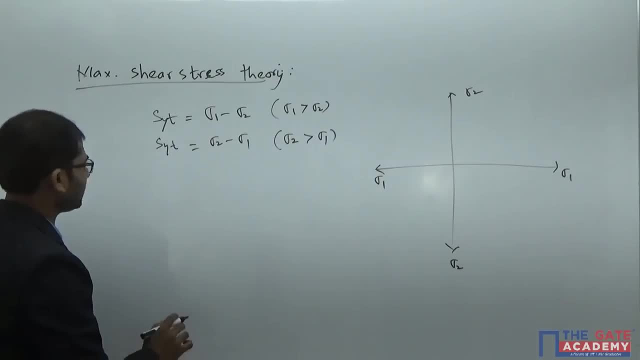 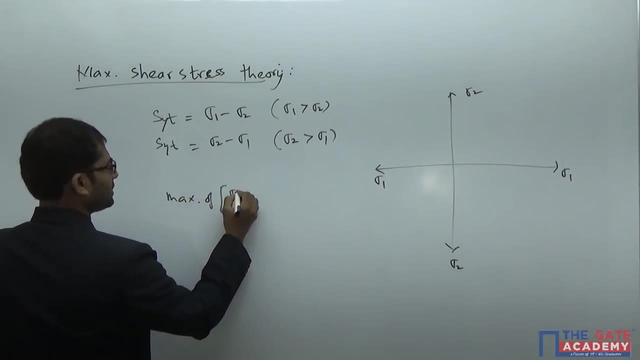 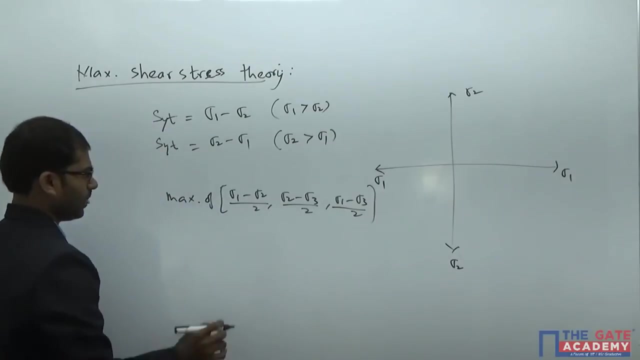 And also if you take 3D state of stress. So what happens is in a 3D state of stress your equation number 1 will change because your maximum shear stress will be maximum of sigma 1 minus sigma 2 by 2, sigma 2 minus sigma 3 by 2, sigma 1 minus sigma 3 by 2.. It is equation. 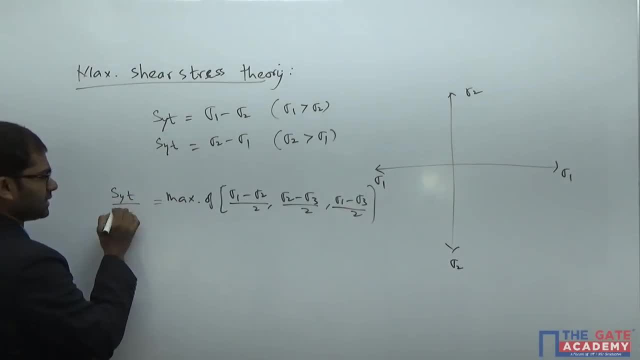 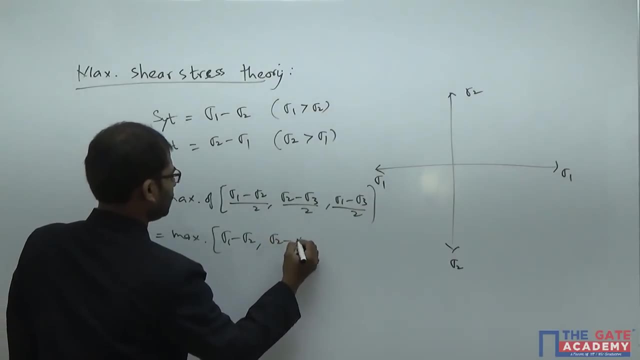 So this should be equal to maximum shear stress in uniaxial case s y t by 2 here. So this equation will be this: maximum of sigma 1 minus sigma 2, sigma 2 minus sigma 3, sigma 1 minus. 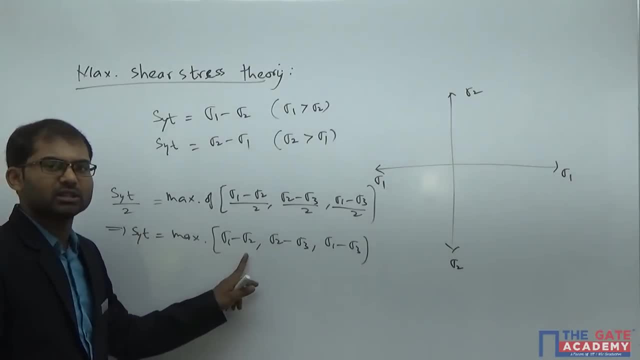 sigma 3.. So, anyways, if you take, sigma 1 is highest value, sigma 2 is infinite value and sigma 3 is the least value you will be taking. this is the highest value out of these 3 values here. But anyways, just write down this way: 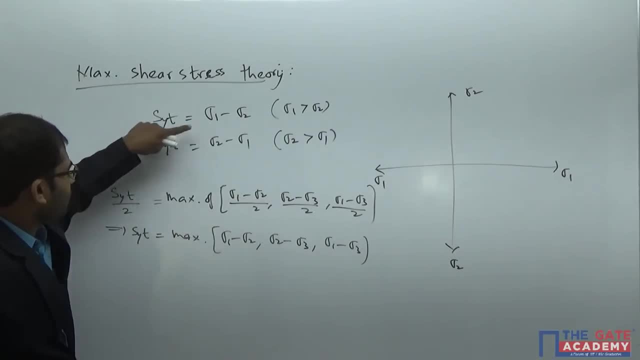 So you will be getting the answer according to this one here. So s y t is equal to sigma 1 minus sigma 2, sigma 2 minus sigma 3, if it is a 2D state of stress condition here. 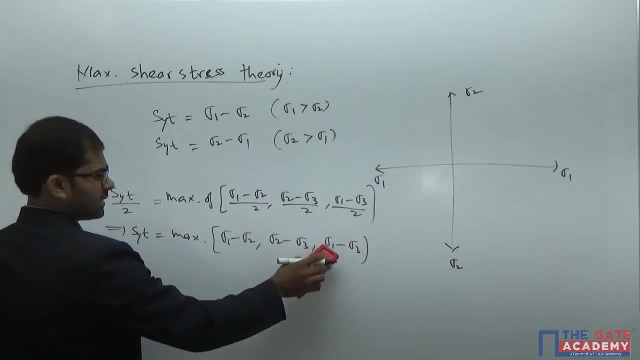 If it becomes 3D, which of the highest value will come? So you can have a chance of sigma 1 minus sigma 3, sigma 2 minus sigma 3 also, But anyways, in this graph you are not plotting. 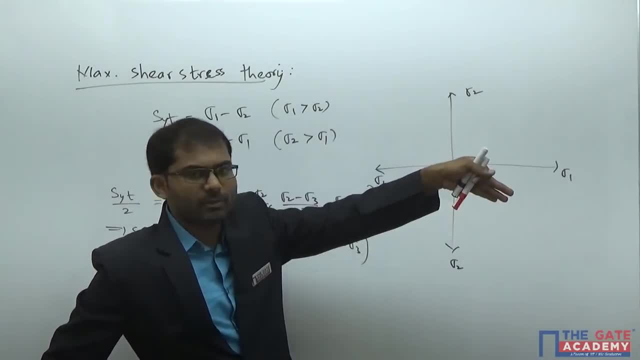 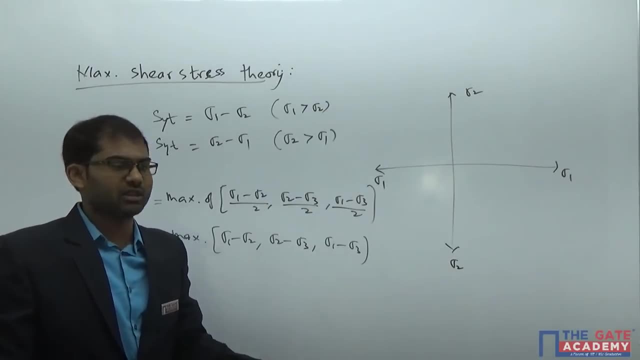 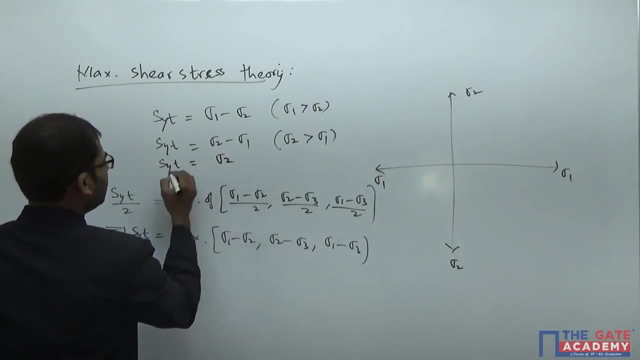 according to sigma 3 dimension. Because if you are plotting sigma 3 dimension also, then it will become a volume, not the region of safety. it becomes a volume of safety there. So sigma 3 will be neglecting here. So your other two equations become: s? y t is equal to sigma 2, s? y t is equal to sigma. 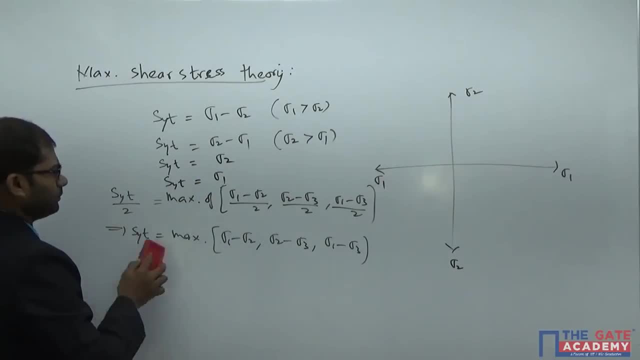 1. These are all the equations here. I am writing this equation here. Just keep in mind that for a 3D state of stress, this is the equation number 1.. So for 3D state of stress, this will become the equation number 1.. So whenever question comes, you just have to. 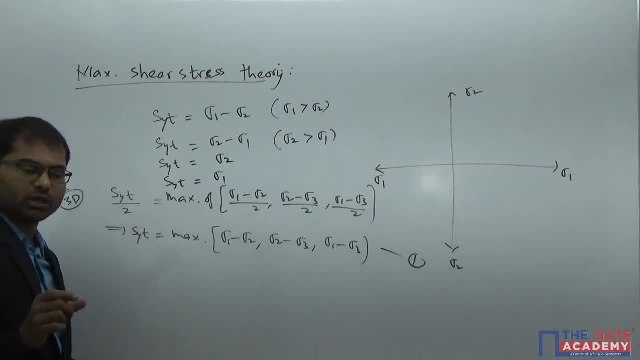 identify whether it is a 2D state of stress or 3D state of stress. Otherwise, if you are going for calculations of 3D state of stress with a 2D state of stress or vice versa, you will be ending up getting wrong answer. So you will be getting the wrong answer, So. 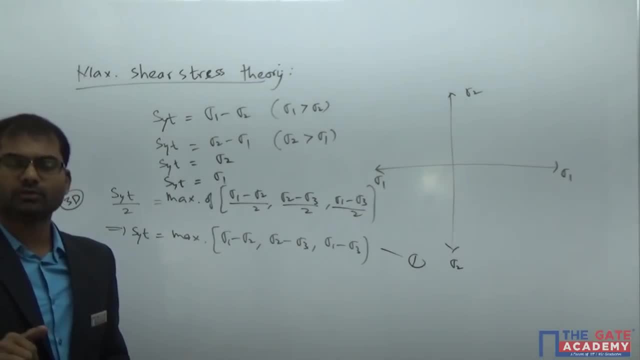 many previous grade questions are there which are given in the play itself. So you should be able to identify whether it is 2D or 3D and apply the correct formula. So if it is 3D, go with this formula. If it is 2D, you go with the earlier formula there. So you 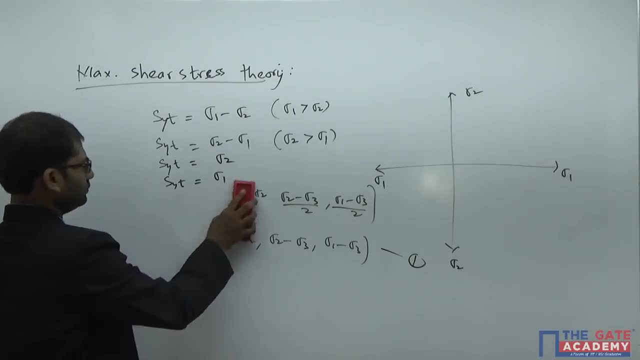 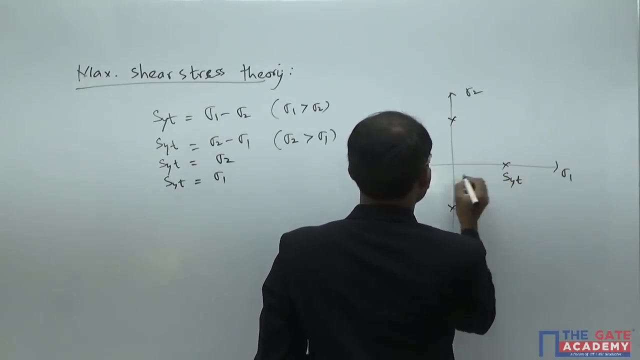 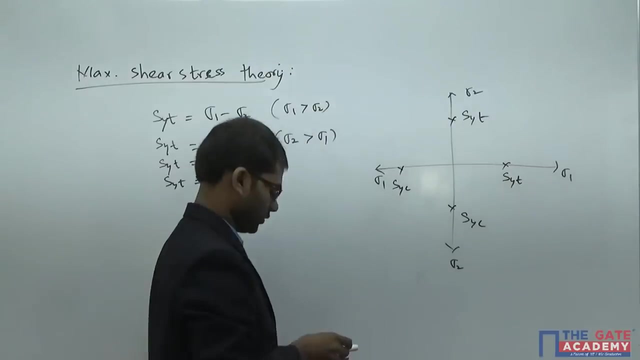 got these equations here. So if you take down or if you plot down these four equations, basically s y t, s y c, s y t and s y c, So anyways, whatever the four equations, we took this 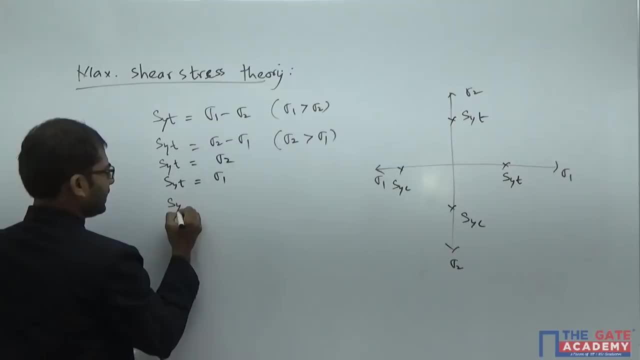 is all there, because here sigma 1, sigma 2 are there. If we take in compression, s y c is equal to sigma 2, s y c is equal to sigma 1.. So these four lines I have already. 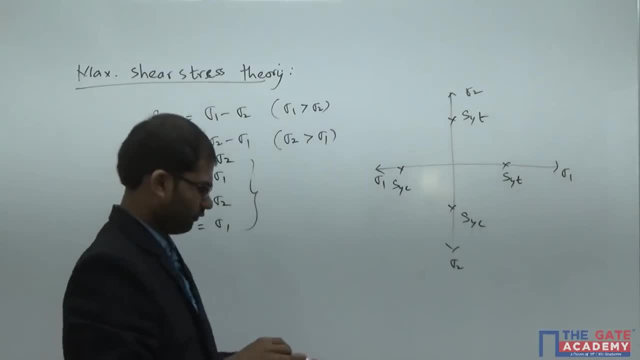 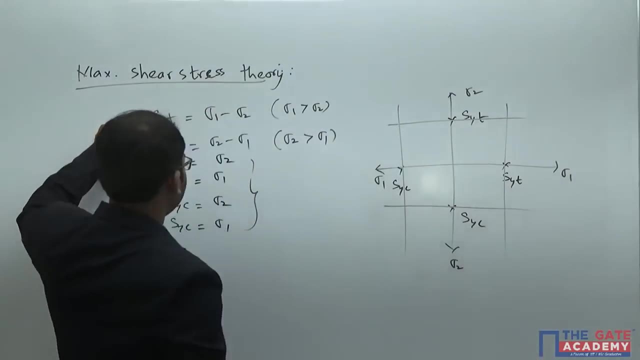 drawn in the previous theory of failure. So they are nothing but vertical and horizontal lines passing through s y t and s y c here. Now, if I want to plot these first three equations, they are actually these two lines here. So the actual region of safety is nothing. 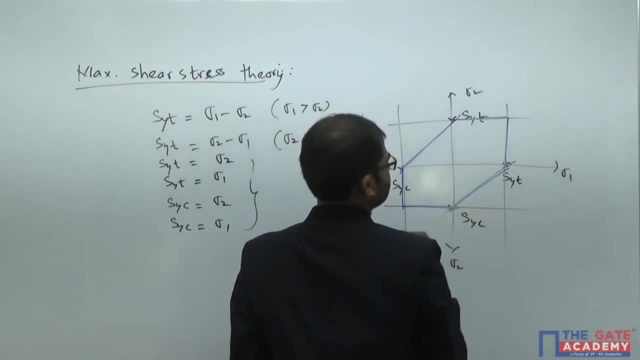 but hexagon here. So if they are coming inside this region, the material is going to be safe. If they are coming sigma 1, sigma 2 values are coming outside this region, the material is not going to be safe. Sigma 1, sigma 2 values are coming out of the region. the material 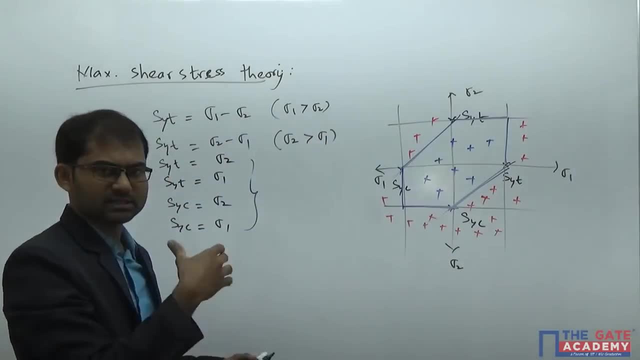 is not going to be safe. So just, I am applying the same concept again and again and deriving equation number 1, equation number 2 and regional safety and getting the answer here. So you take any question from previous gate papers. So you just have to evaluate whether the factor of